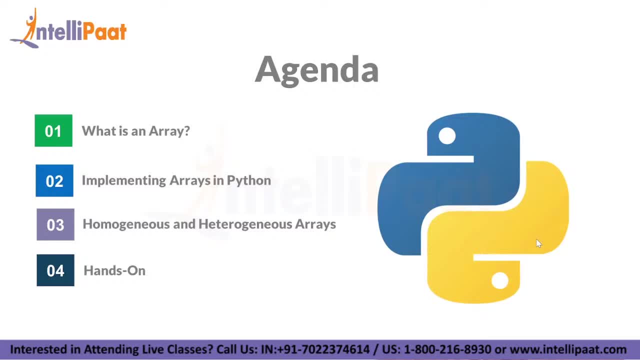 then we will discuss the Python array module to work with arrays Moving further, we will discuss the CRUD operations on arrays using Python And finally we are going to sum up this session with NumPy arrays. I hope the agenda is clear to you guys. So 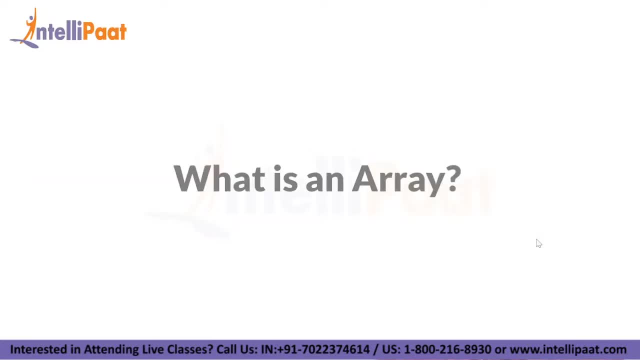 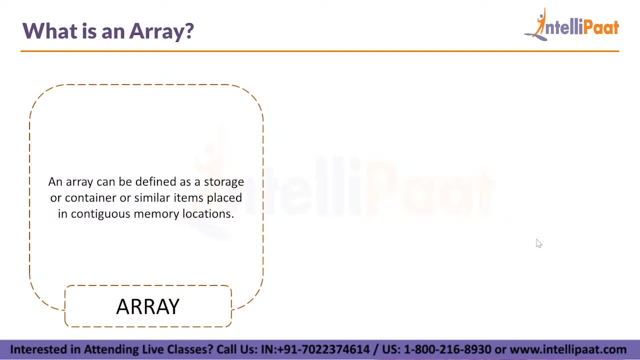 without any further ado, let's begin. So what exactly is an array? We can consider an array to be a storage or a container that will store items of similar type. These items can be retrieved later for any computations. These elements are stored consecutively in. 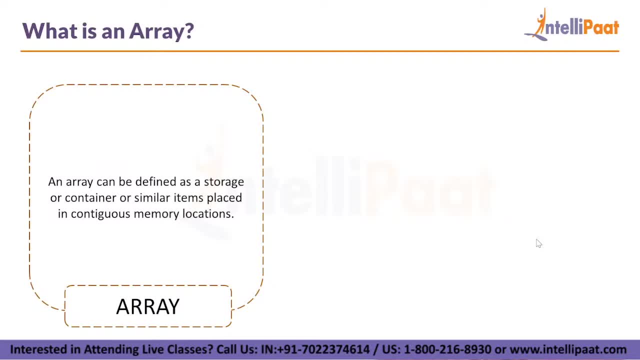 the array and can be identified with the indexes assigned on each of the elements positioned in the array. These items can be of any data type and will follow the indexing for retrieval of the elements. Creating, adding and removing elements from the array are the primary operations. 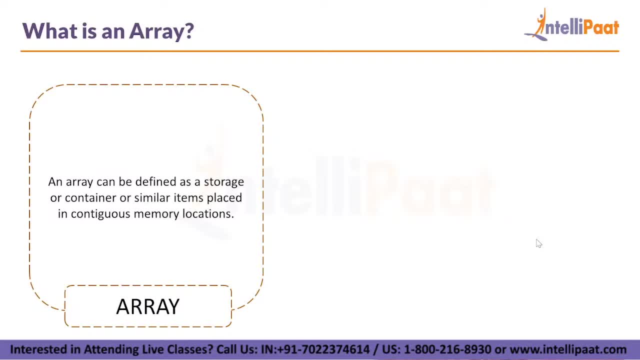 that you must familiarize yourself with, And all the other operations are built on top of these three operations. only A simple analogy to explain how arrays work is how you stack books on a shelf. Now, you would want a shelf that would store all your books. 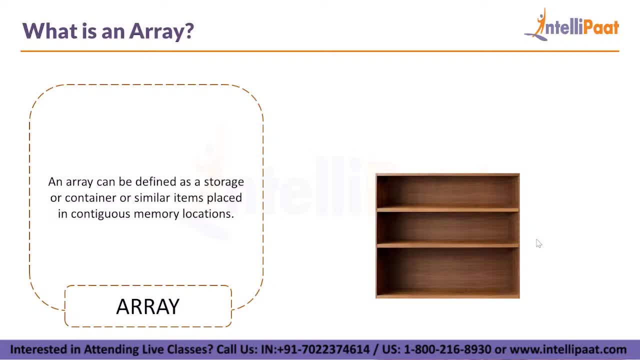 So this is exactly like an array. You should be able to get the books from the shelf without searching through it all, And there has to be a system of stacking the shelves So you can stack the books with the same numbers or, you know, with the same genre or books starting. 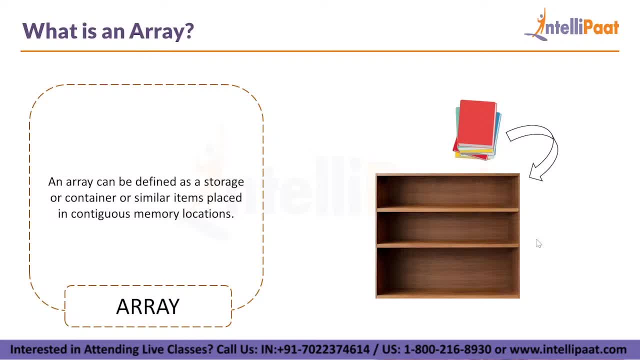 with the same alphabet, etc. So you can stack the books with the same numbers, or, you know, with the same genre, or books starting with the same alphabet, etc. But the shelf will only contain books. And now that we have a basic idea of what exactly, 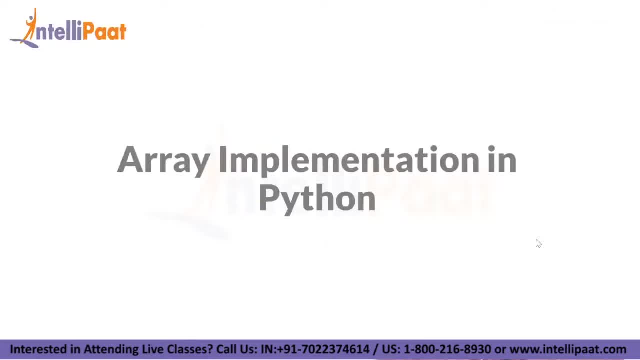 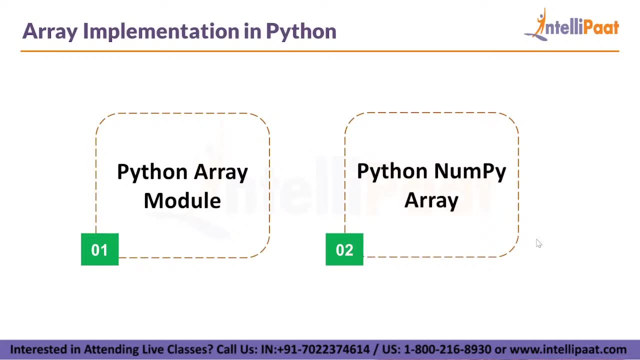 is an array. let's see how we can implement them using Python. To implement arrays in Python, we can follow the following approaches: First is using the list, and then we have the Python array module and the Python numpy arrays. So to understand how they will differ, let's 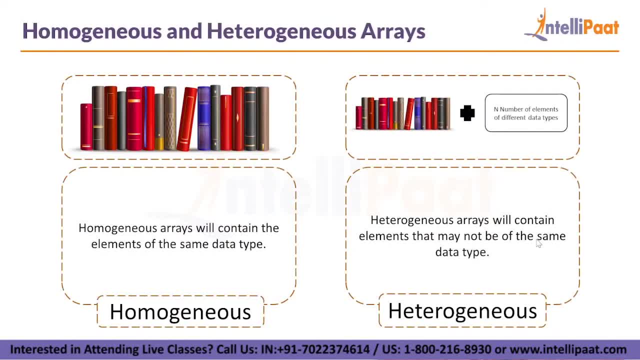 understand the concept of homogeneous and heterogeneous arrays. So what exactly are homogeneous and heterogeneous arrays? The easiest way to differentiate between a homogeneous and a heterogeneous array is that the one that contains only single type of elements will be homogeneous, and the other that can store elements with different types are known. 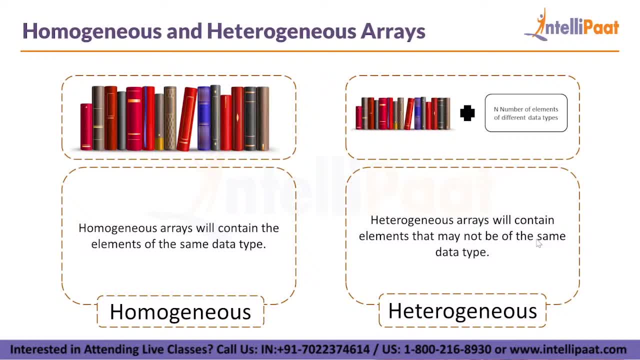 as heterogeneous arrays. The implementation of arrays with Python array module and the Python numpy only allows homogeneous elements to be a part of them, while the list can store heterogeneous elements as well. And now that we have a basic understanding of arrays, let's move on to a few examples to understand the array implementation in. 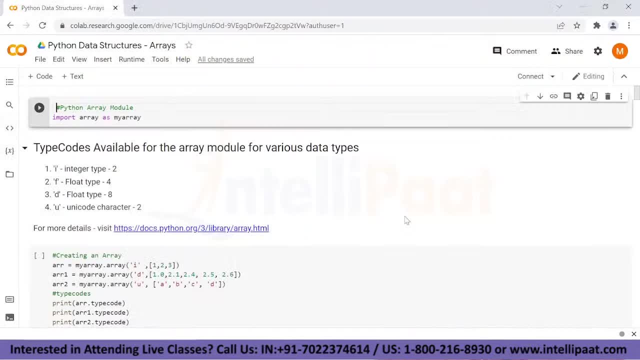 Python. So first of all, we are going to start with the implementation of arrays using the Python array module. Now, to start with that, we have to first import the array module using the statement import array, and the alias we're using over here is my array. 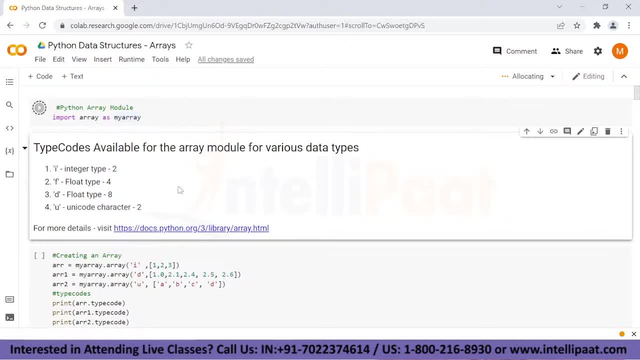 Before we start we have to understand there are type codes available for the array module for various data types. For example, if you're using the integer data type, there's going to be another type code. For float, there is another type code, and for Unicode characters separately. 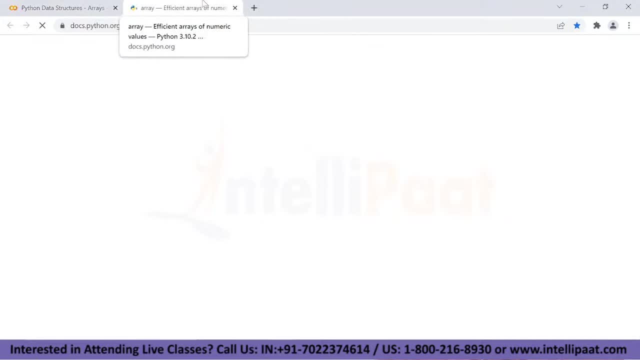 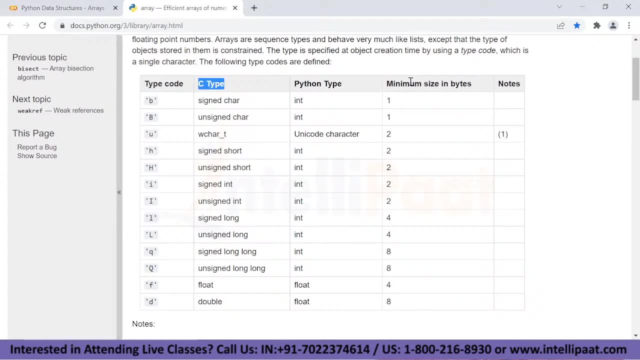 Now to discuss more on this, we can go to the link available over here, which is official documentation. Here you can see the type codes are given for C, for Python, and the minimum size in bytes is also given. So since we can see in the Python types it's mostly integer and the float values available. 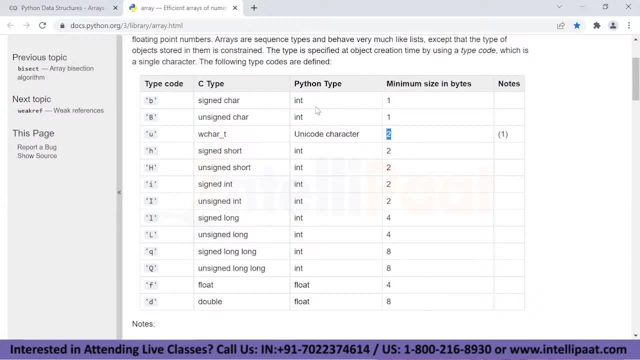 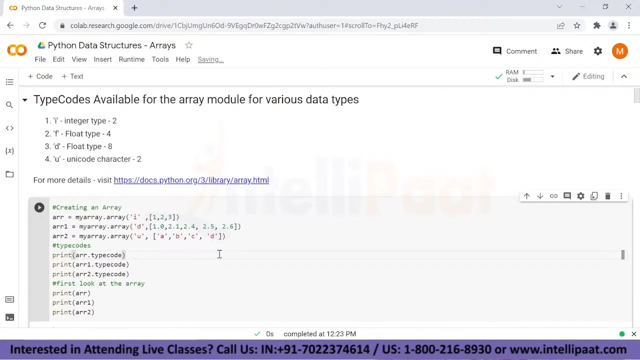 with the Unicode character. Number of sizes available is two in bytes And for, let's say, integer, signed integer, we have two, then we have float four bytes and for double it is eight. First of all we have to understand the basic operations we have to do inside an array. 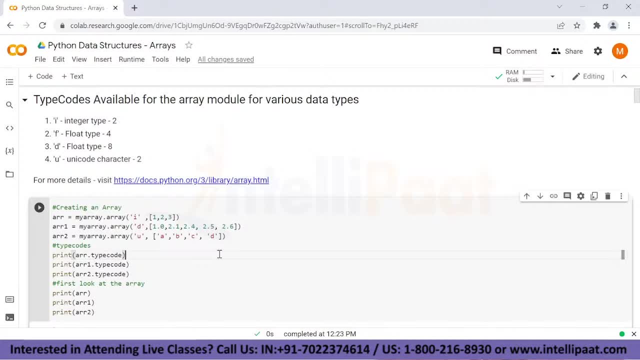 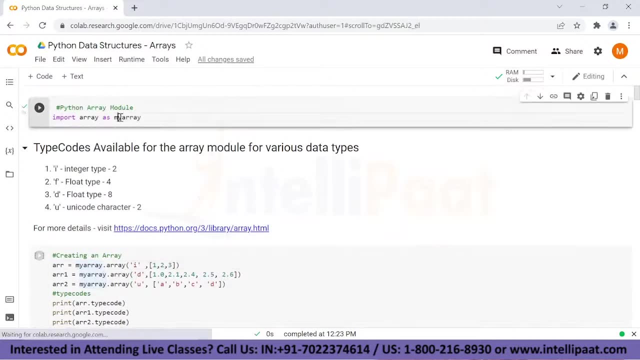 which is creating an array. then we have to add elements and removing the elements from an array. So, starting with creating an array, we can use the Python array model, which we have imported from this statement, and, using the alias, we are creating the array we're providing. 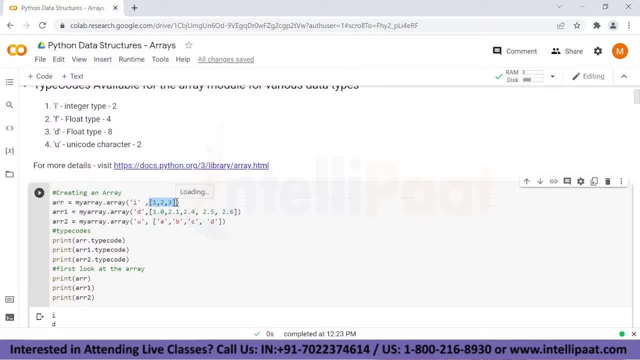 the type codes and inside a list over here we are mentioning the elements that we want in our array. Similarly, we have another array, arr1, and then arr2.. So we have to create an array. So we have to create an array. 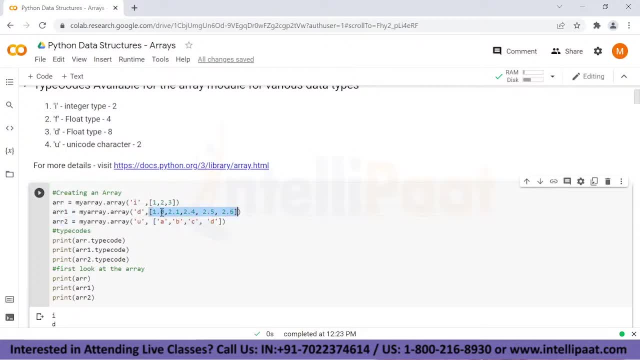 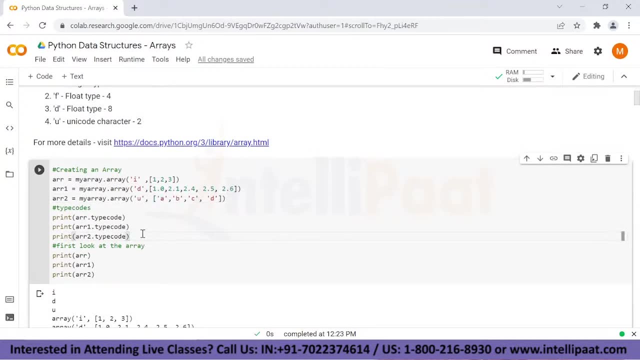 So right now we have two with separate values. One has the floating point values with the type code D, and for the Unicode characters we have the type code U. Now to check the type code we have a method called type code, So we can print the values using the type code method available from the array module. 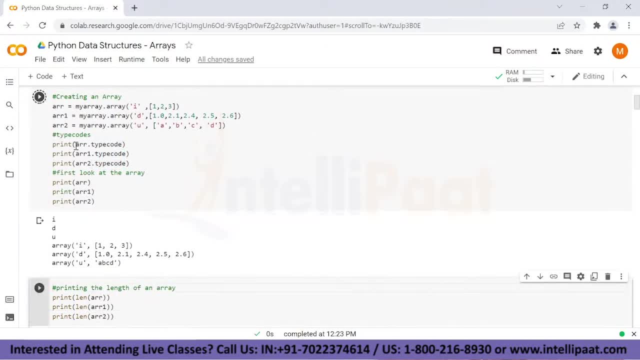 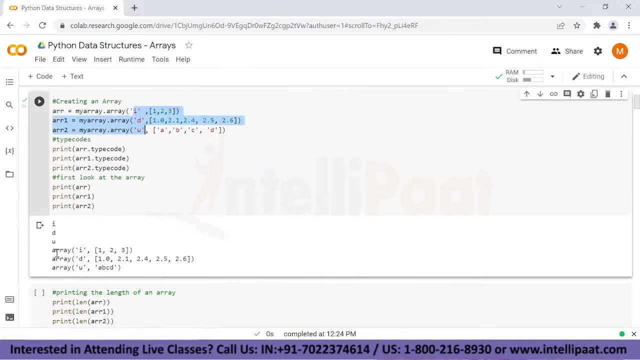 and then again we can print the arrays, which will look something like: So the first print statement is actually giving us the type codes, which is I, D and U, which we have assigned into our arrays over here, and the next values are giving the array with. 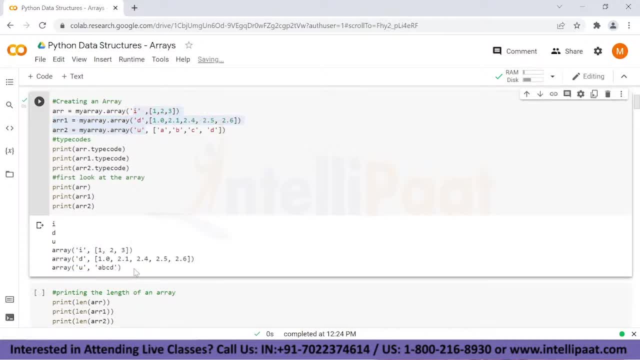 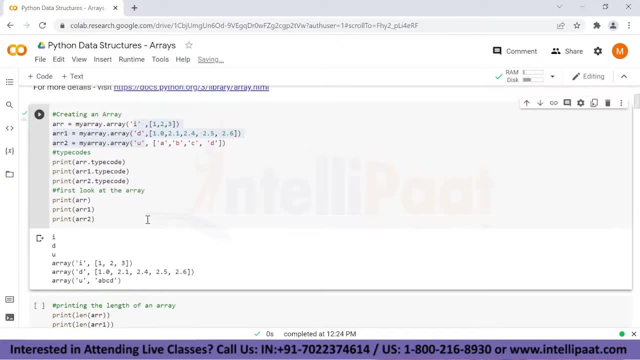 the type codes. Now, this is not exactly how we want our elements to be accessed, So that we'll discuss later on in the session how we access the values inside an array. But before that, there is another very important section where you have to understand how you 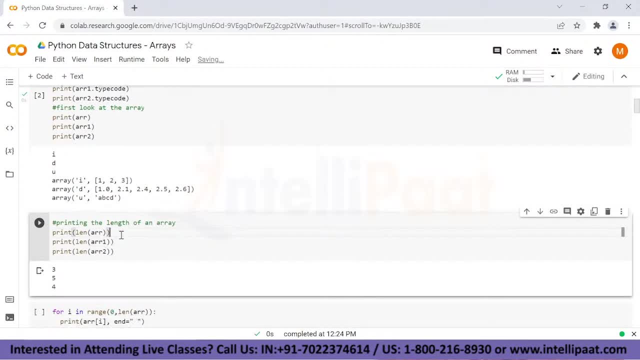 get the length of an array. So whenever we are computing any value, let's say accessing values or removing elements, we have to understand how we access those elements. To do that, we have to make use of the indexing part, which we'll discuss just now And before that. 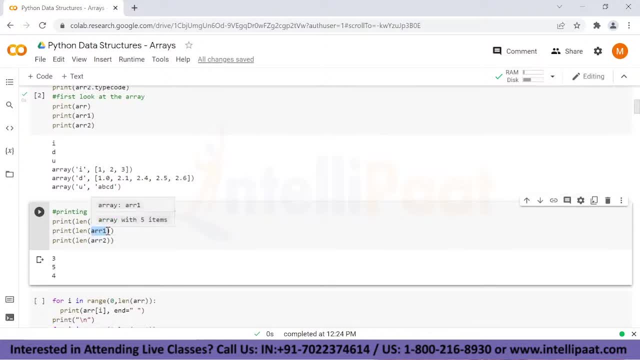 we have to understand the length of an array, because until unless we are aware of how many elements are placed in the area or what the length of the array is, we cannot specify the range in which we want to iterate over. So iteration basically takes place for accessing. 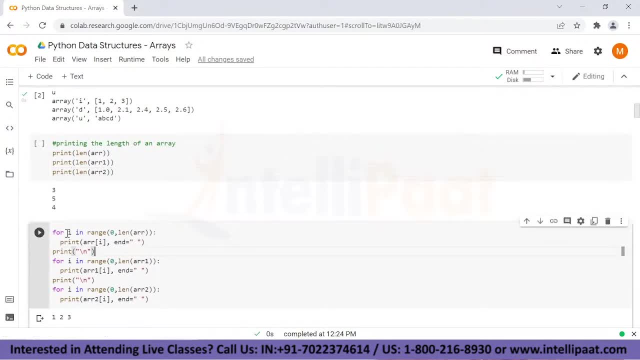 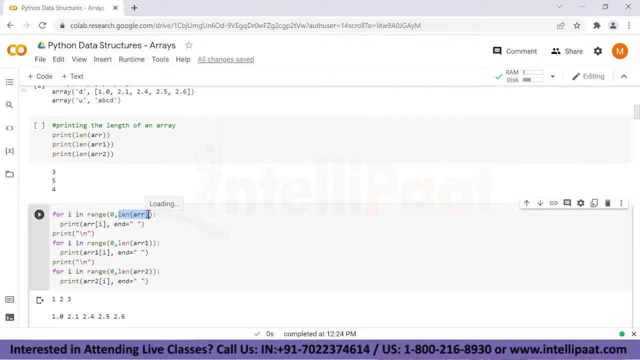 the values or basically printing the array. So here we have done just that. we have used the for loop, which is in the range length of the array. Now, if we already know the length of the array, for example if it's six or five, we can put: 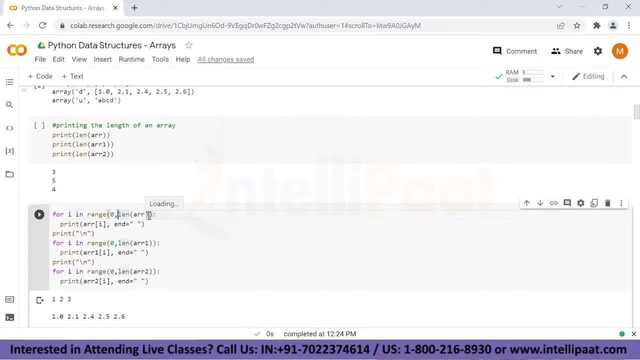 the range over here as five or six, But for cases where we have the array in the length of 1000s and 10,000s. we don't want that, So we'll just use the length method over here to get the length of the array. Now, for every value inside this range, it will print the 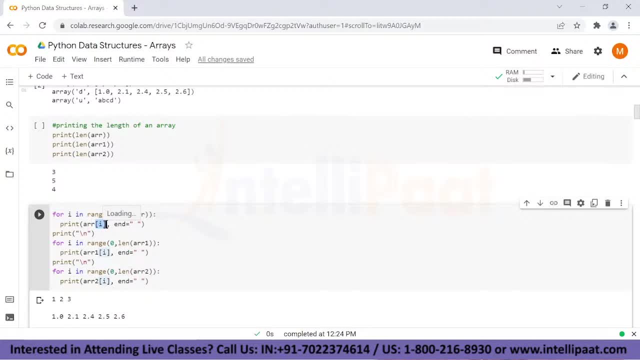 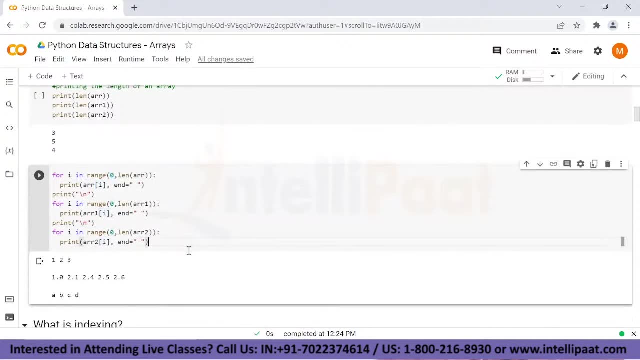 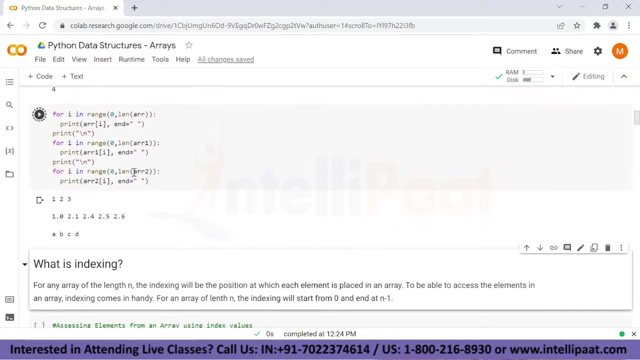 index value or whatever element is positioned at that particular index. Now we are starting from the range zero, because the index starts from zero. Now we'll discuss that just in a while. So, just for example, here is how we get the values from the arrays we had just created. So when we run this code, this particular code, we 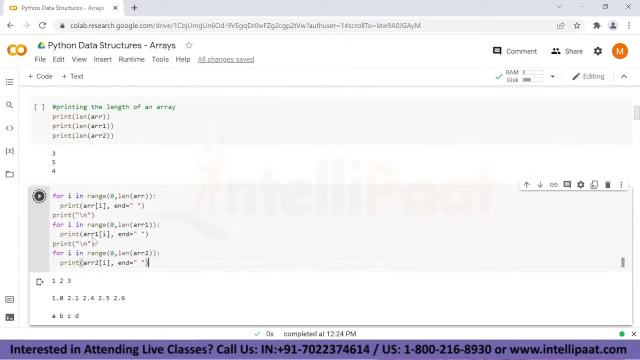 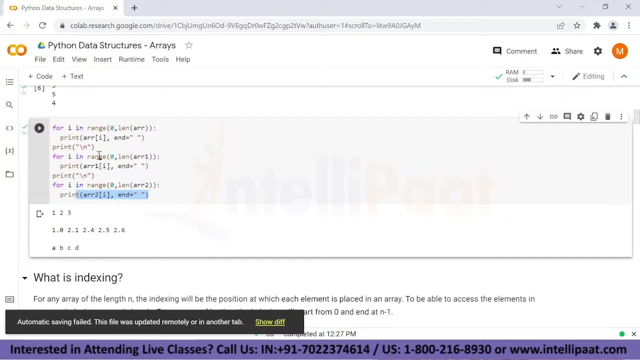 are getting the values as one, two, three and so on for each of these arrays that we had already assigned. Alright, so we are getting these elements, or the elements from an array, from each of the arrays: array arr1 and arr2.. So this is how we create an array and display. 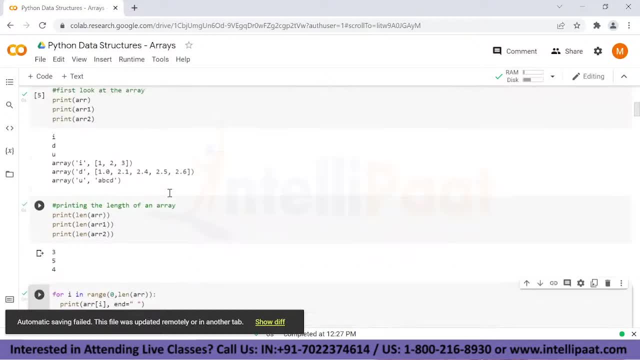 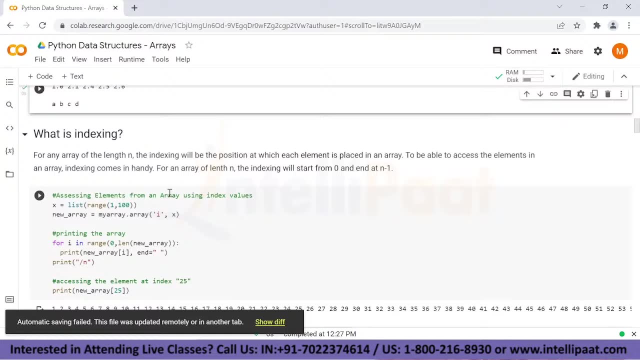 those values using a for loop. Now we have already discussed the length of an array, And we'll discuss so. for any array that is of the length n, for example, the indexing will be the position at which each element is placed. the index elements will start from zero and go until the end of the 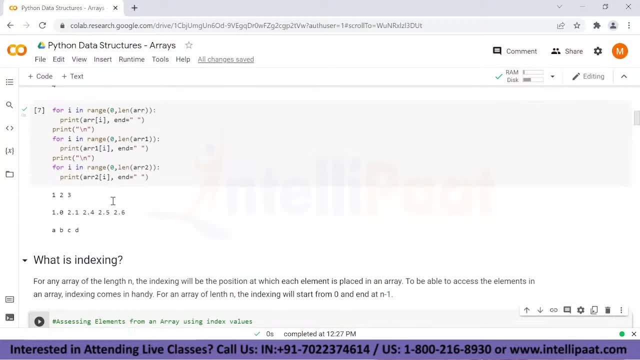 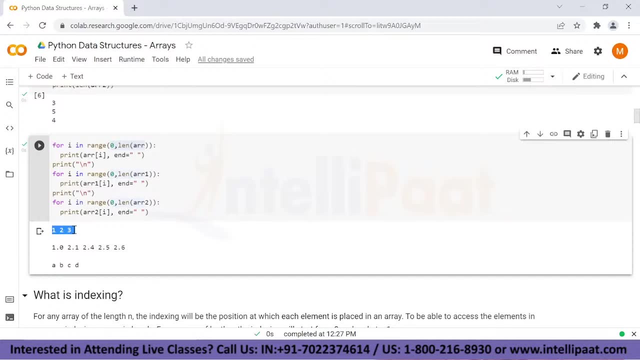 array minus one. So, for example, let's say we have an array over here which started from one, two and three, only has three elements, but the index value will be zero- one and two- because the index is starting from zero and going until the end of the array, So that 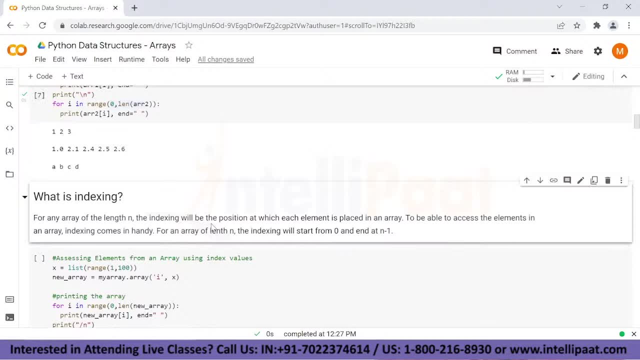 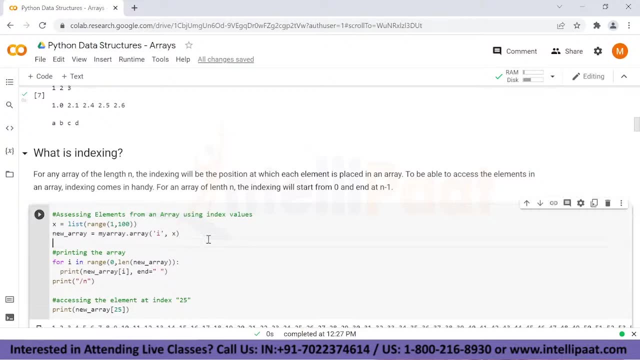 is the only significant part of indexing which we have to remember that it starts from zero, So automatically we have to understand that the entire length of the array minus one will be the entire indexes that we have for the array. Now coming back to how we can. 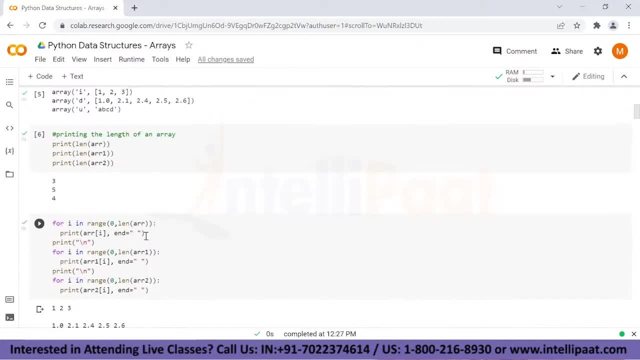 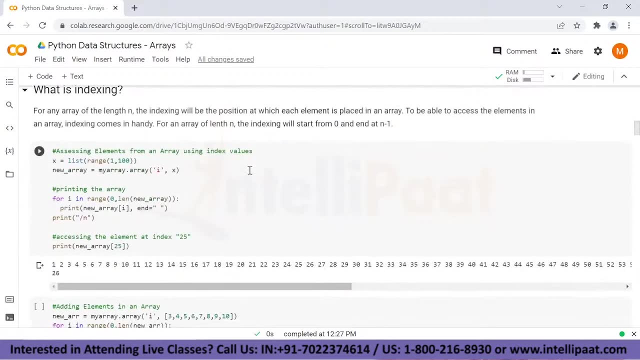 access the elements from an array using index values. This is how we can do that, just for how we have done over here, just providing the index value, whatever element we want to be displayed at Now. here we have an array which is a list in the range one to 100, basically. 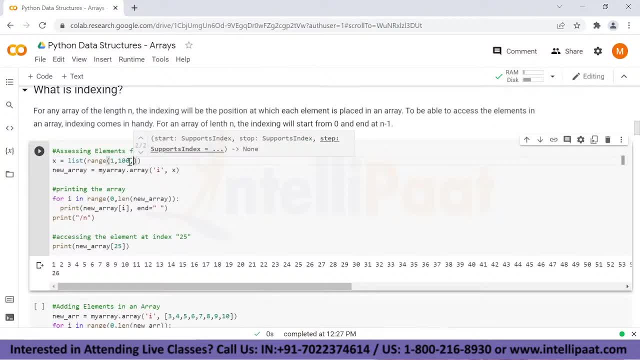 has hundreds of elements. So we have an array which is a list in the range one to hundreds, has hundreds of elements. Just to be a little bit clear over here, what we can do is add a step of two over here so that we'll have only 50 elements now. Now, after this, we have 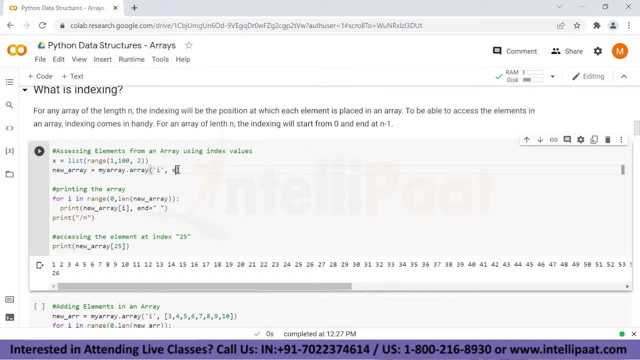 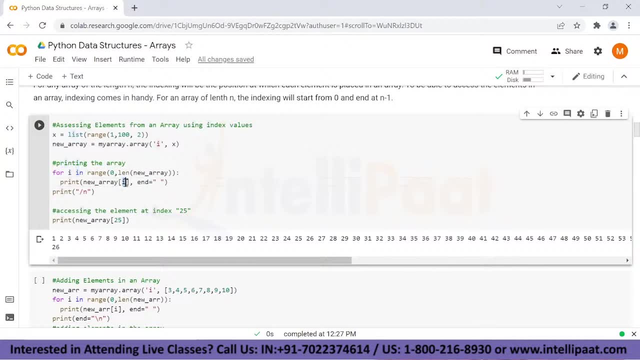 created a new array with the type code I and provided the list over here which we have created just now. After this, to print the array, we are using the for loop again, So we are getting the arrays from the index value which we have iterated over from the range. 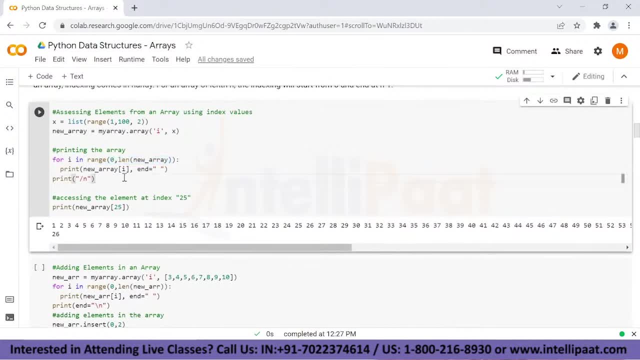 of length of new array. And this is how we get the array. Now let's say, if I want the value which is at the index number, let's say 25. Or probably at 26 or 27. So that's how we get the values. So this is a very basic example. 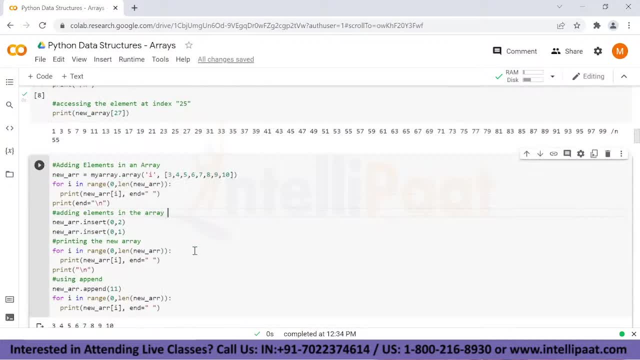 of how you can access values or elements inside an array. So now comes the part where we add the elements into an array using the Python array module. First of all, we create a new array. Inside this, we have all these values And we print that array again. So this is. 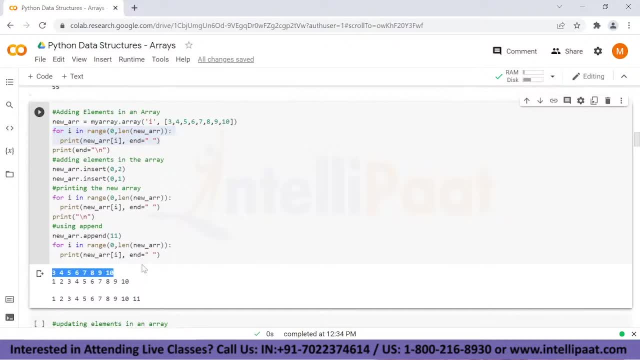 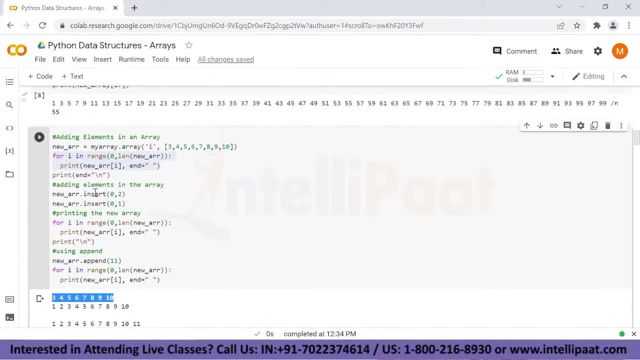 the array 3456789 and 10.. Now we want to add new elements to it. There are two approaches to this. You can use the insert method or you can use the append method. By using the insert method, you basically provide the index which you want to place your element at the new element. 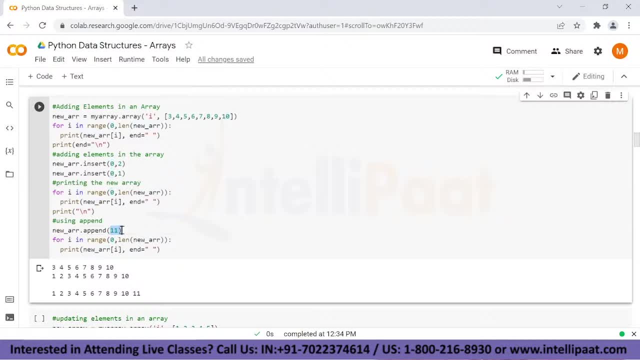 And after this, the append method is basically going to append or add the value or concatenate the value at the end of the array. Now, when I insert 2 and 1 at the 0 index, I get the value as 1, 2 in the beginning, which is the 0 index, And after this, if I append value, 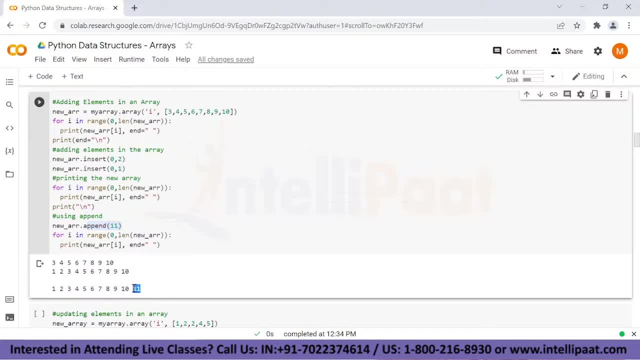 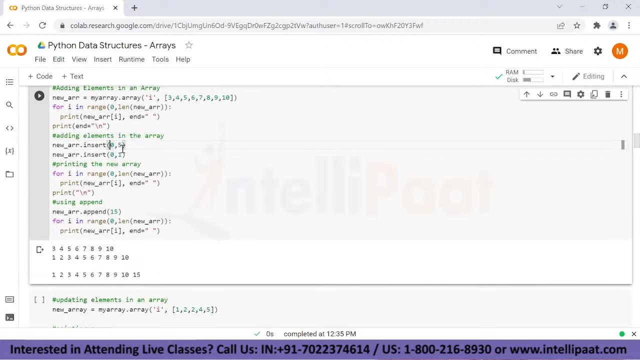 which is 11,. it's just going to add the number 11, or the element, at the end of the array. Now, to understand this, let's just change these values. Let's say, if I want to add 15 at the end of the array, it will be 15.. And instead of 2, let's say, if I want to put 5 at the 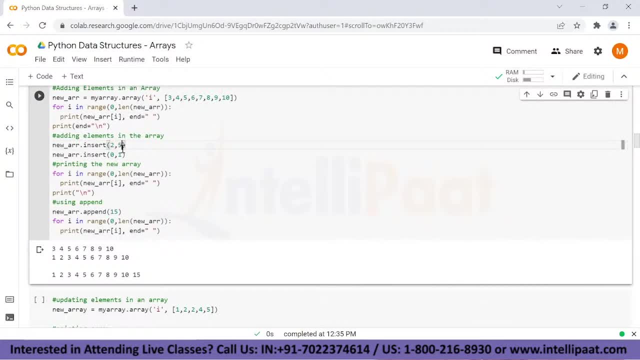 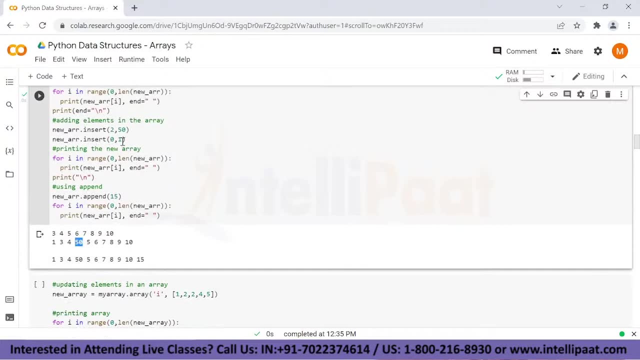 index number 2, or instead of 5, we put 50 over here. So the value will be 50 at the index number 2. And after that at the 0 index we're adding again 1. So if we comment out, 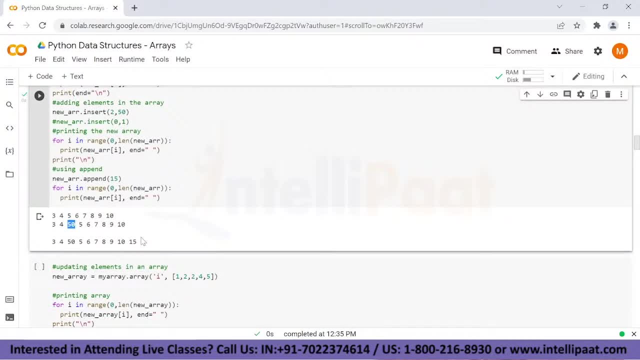 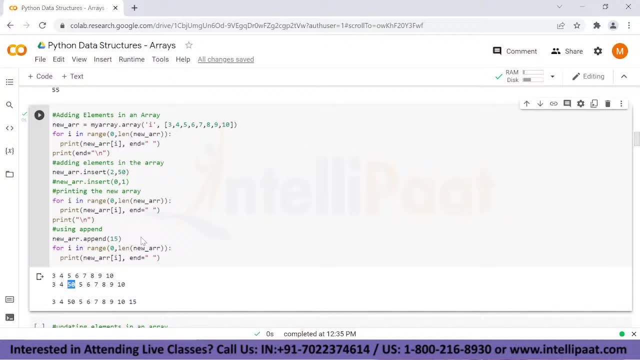 1,, you'll see that at the index number 2,, we have added the 50. So that is how you simply just add the elements into an array, And this is how easy it is. With the Python programming, it basically becomes a lot easier to deal with any data type, be it array, if it is. 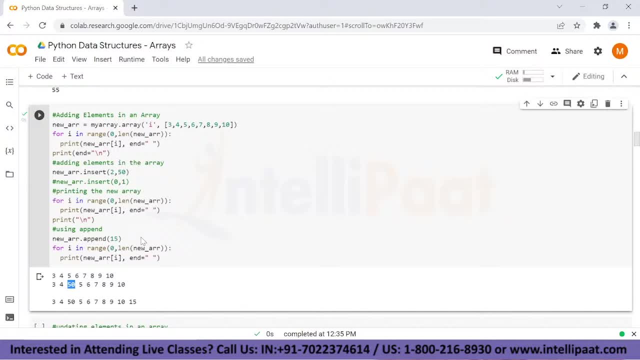 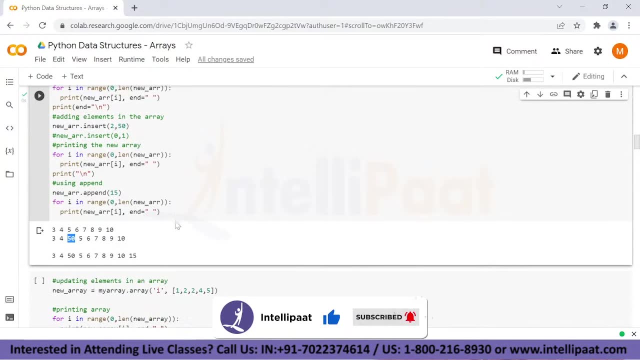 a linked list or any other data structures that you want to talk about. Python actually makes it pretty easy to work with just that. you have to understand how the logic works. So basically, you have to understand the addition of elements and removing of elements as well. 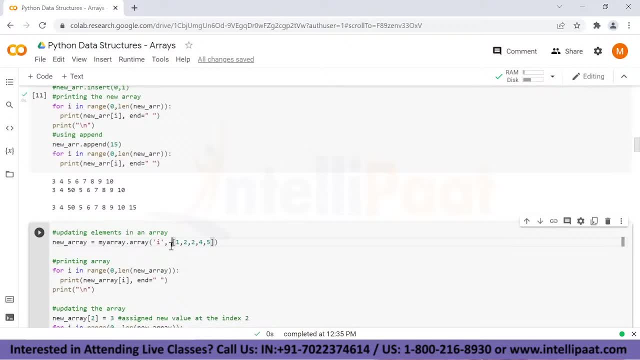 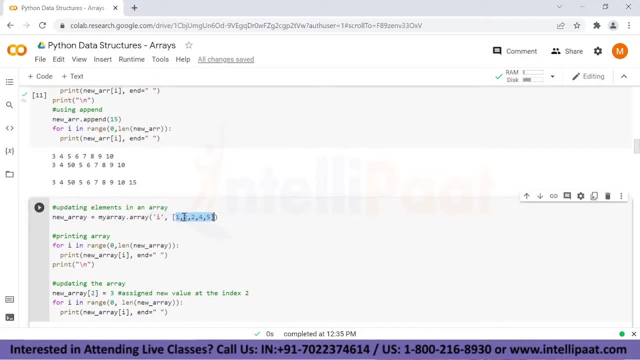 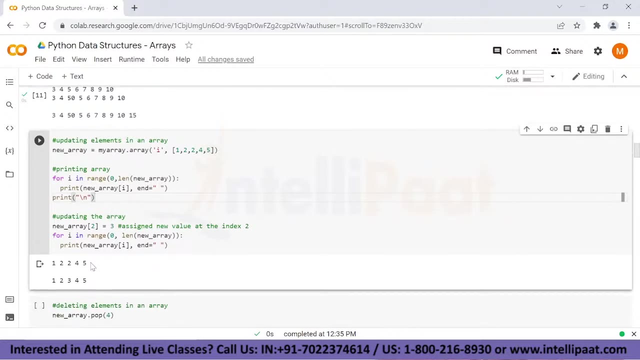 So, moving on, let's talk about how you update these elements inside an array. For example, we have this array which has 1, and 2 is actually twice in that array. So now I want to update 2 into an element which is 3.. First of all, we print the array, So this is the array. 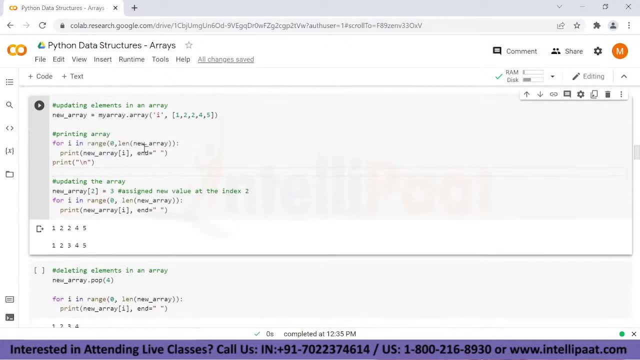 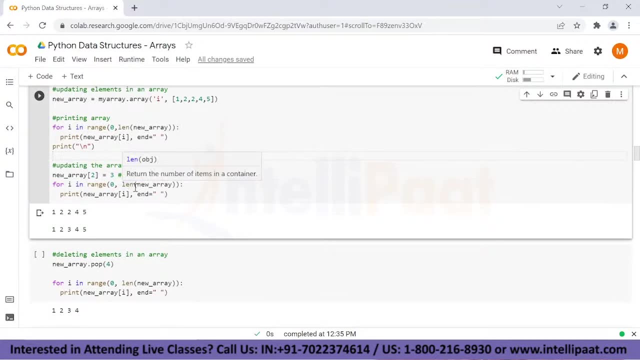 resulting array And we are using the same approach: the for loop and the length of the array After this to update the array. basically, what I have done is accessing the element at the index number, which I already know, And after this I update this value to 3.. So this is how I have just done it, assigning 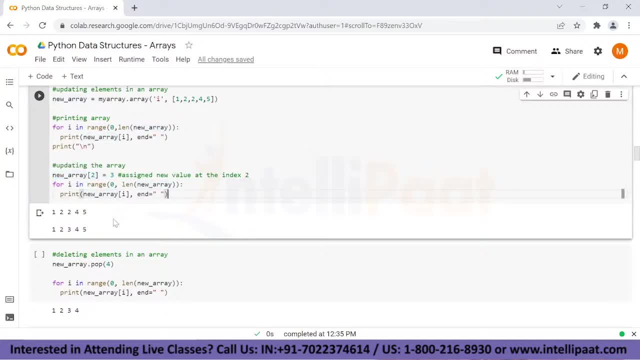 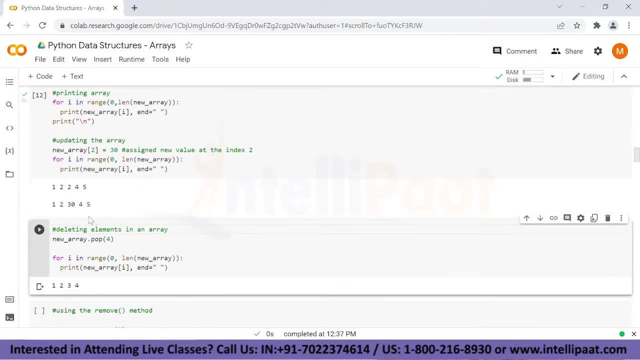 the new value using the assignment operator, And then when I print the array again, it is updated. Now to understand this again: instead of 3,, let's say if I wanted to put 30 over here, the value will be updated with 30. And instead of this, let's say: if I wanted. 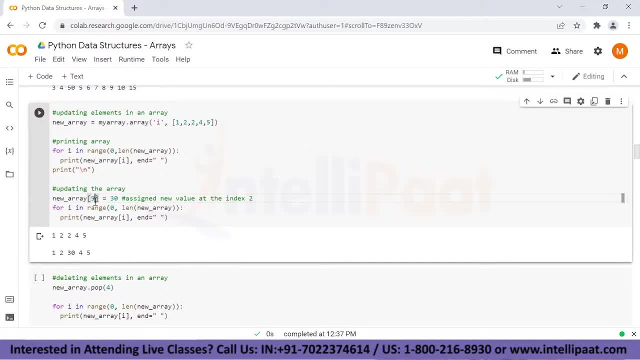 to put it, at the fifth index. so do we have a fifth index over here? Since we only have the five elements, we don't have the index, and it will throw us an error. So let's say we don't have the index and it will throw us an error. So let's say we don't have the. 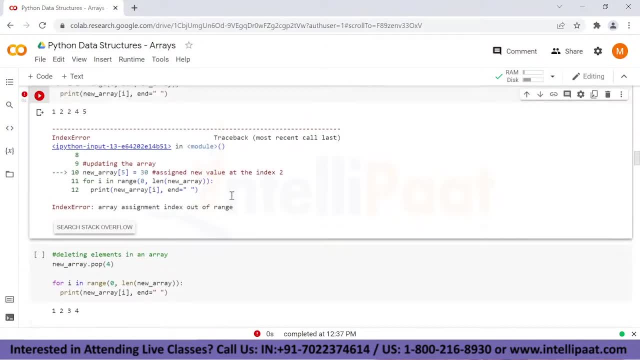 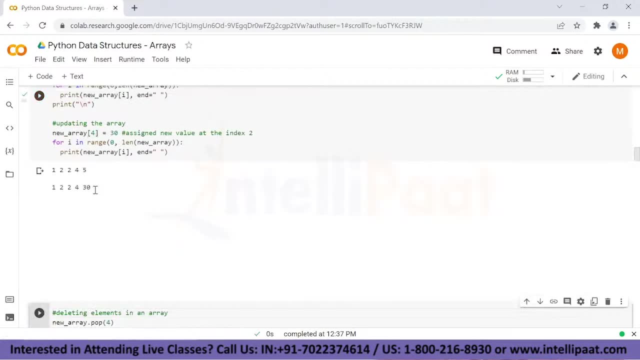 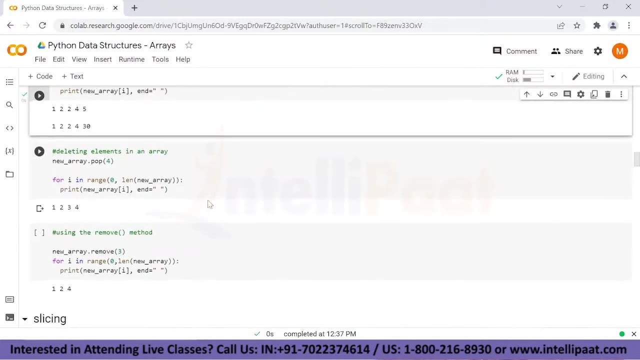 which is assignment index out of range. when you are going out of the index range, it is going to throw you an index error. so that's how you know you have surpassed the index that is available to you in the area. so this is how simply you can just update the elements inside an array. after this comes the part where 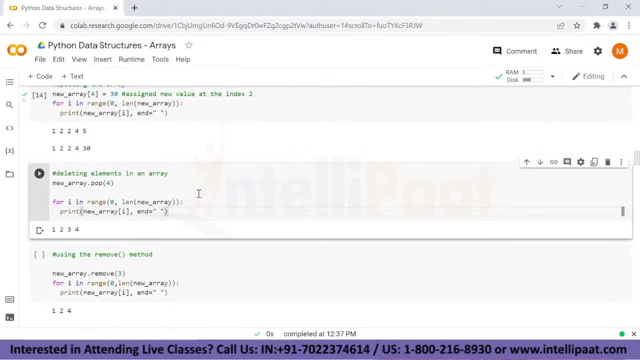 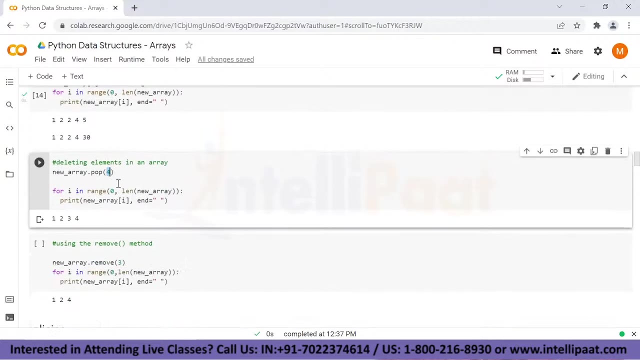 we delete the elements from an array. now, this is basically removing the elements from the array, and for this we can use the pop method. so now, if I wanted to pop for let's say, for example, what will happen: we are basically giving the next value, number 4 over here. so instead of 4, let's give it as 2. let's see what. 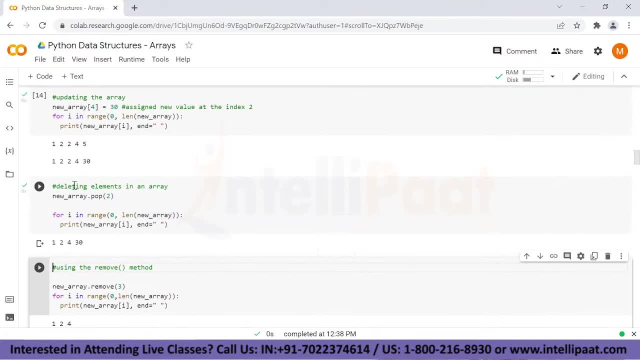 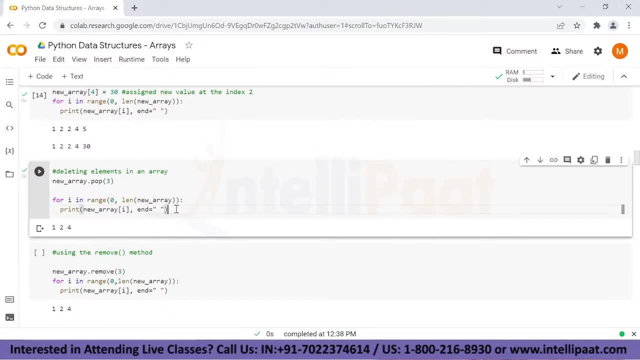 happens. so now we are missing one value at the index number 2, which was 2 over here. now let's see, if I do this at index number 3, what will happen. now we have removed the element at the index number 3 as well. so this is how simply you can. 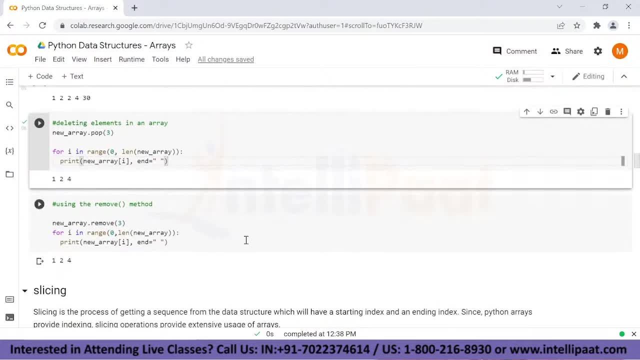 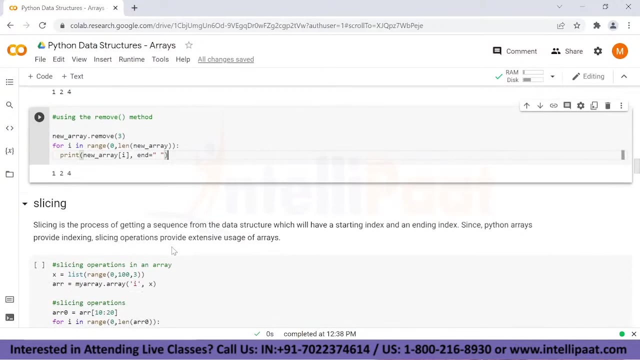 just delete any elements using the pop method. and since we have already covered creating, creating an array using the Python array module, we have updated the values, we have added the elements inside the array and we have learned about how we can delete the elements. now comes the part where I'll tell you about slicing. but so what? 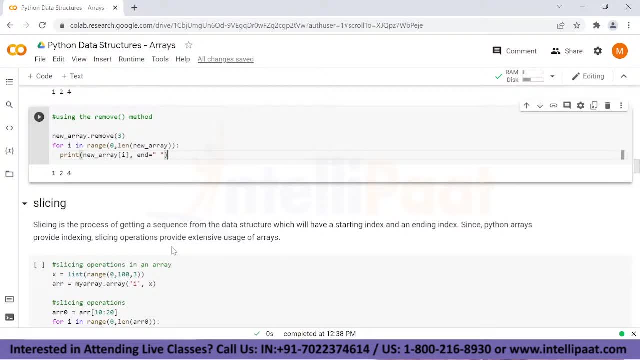 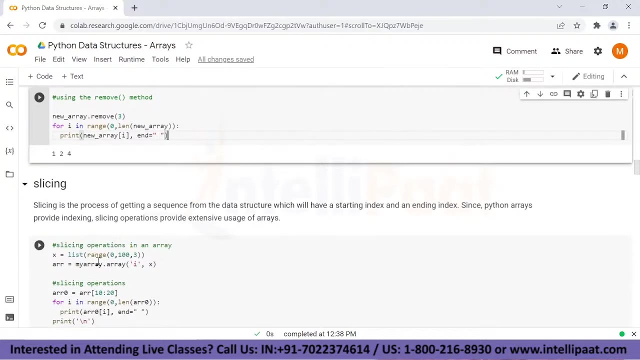 exactly is slicing? slicing is a part of concept which is also similar to how we use indexes. now, in the indexing it is not just one element we can get at a time, we can get multiple elements. so that is how we use the slicing operations. basically, let's say, if I want to get so there's an array X over here which is in the 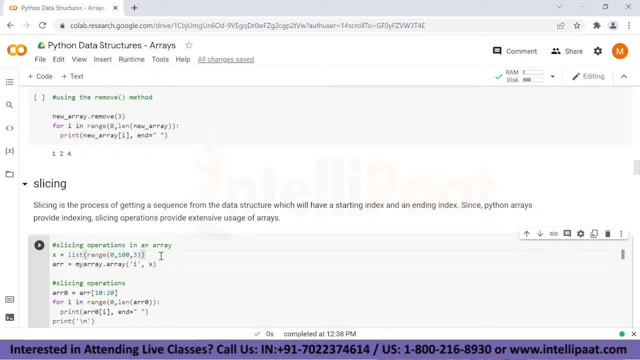 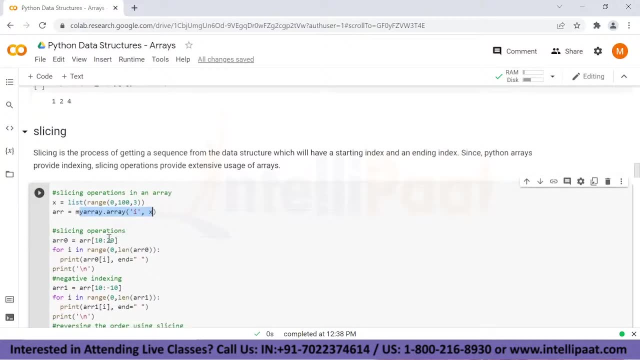 range 0-100 and we have taken the step as three. we have probably thirty three elements inside the array. now, if I wanted to, let's say, only get the first ten elements, or if I only want to get from the tenth index until the 20th, 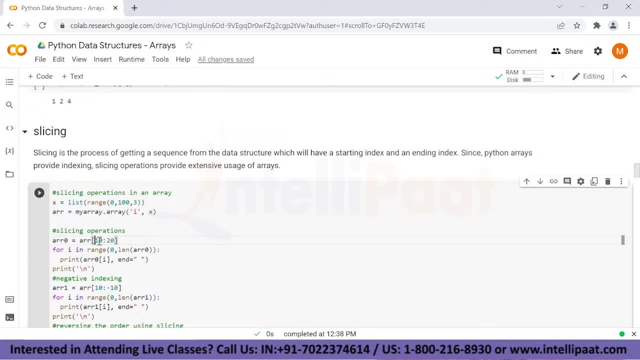 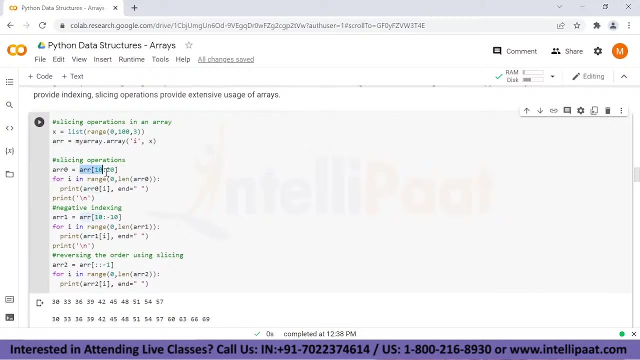 index from the array. so that is how we use the indexing. so inside the indexing we use a colon over here and after this we have the ending index and the starting index. so when I print my new area over here, which I have got from the slicing operation, you will see that this is basically how much values I'm getting. 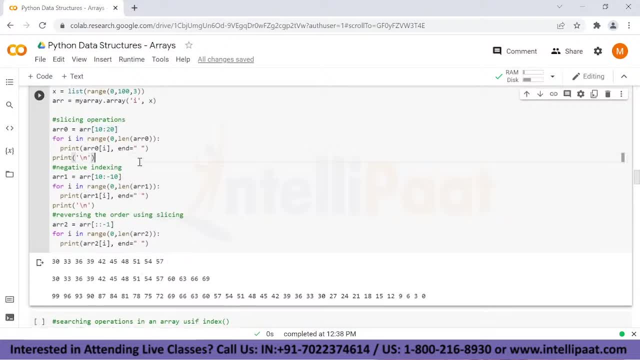 or how many values I'm actually getting. another important concept in slicing is negative indexing- how you can use the negative indexes. so let's say, if I wanted to get, the starting point will be the 10th index and the ending point is minus 10, which is basically the 10th index from the end. and one more thing is: 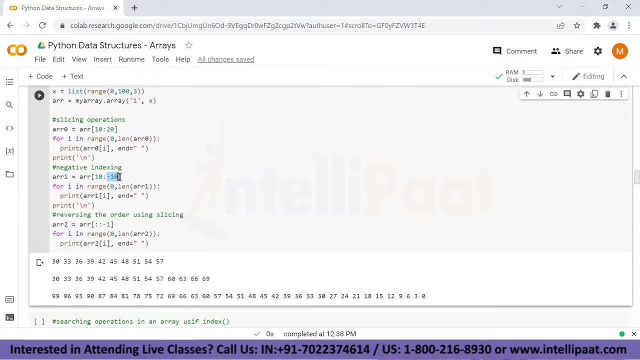 we do not really have back propagation inside the slicing operation, so we cannot go from back to, let's say, to the front. see if I do it like minus 10 to minus 20. so this will throw me an arrow. because we do not have slicing operations, our negative indexing will not back propagate and after this we 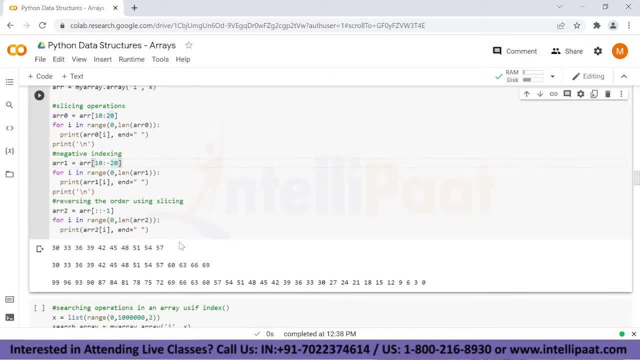 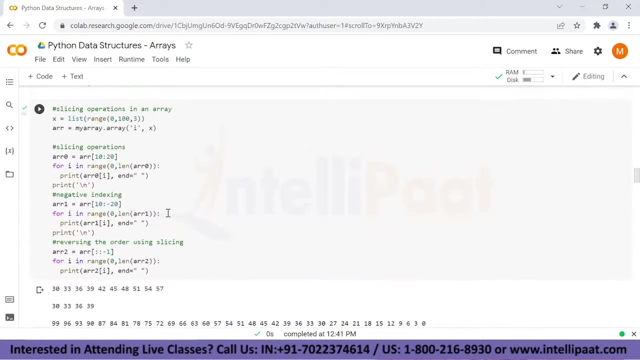 have have another important slicing operation, which is basically reversing the list over here we have used colon, colon minus one, and this is how simply you can just reverse the list without using the reverse method from the list. so this is all about the slicing operations we have and if you have, 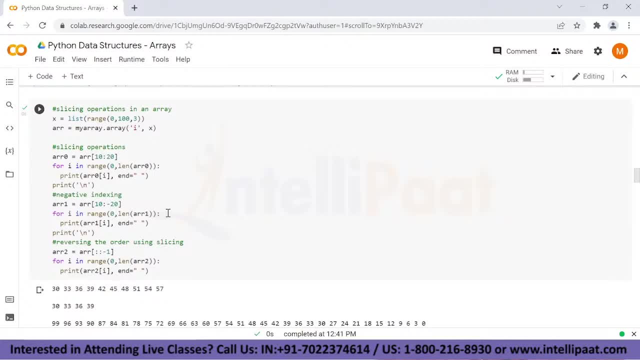 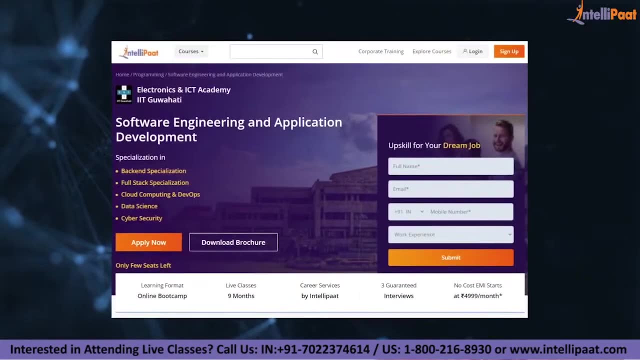 any questions, guys, you can mention them in the comment section below and we will be quick to help you out in any problems you're facing with the arrays. just a quick info, guys. if you want to make a career in software engineering, then intellipad provides an advanced certification. 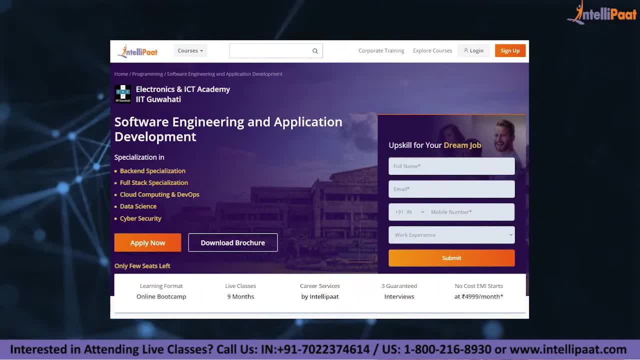 program on software engineering and application development by enict council of iit guwahati and it is taught by iit guwahati professors and industry experts. this course is designed to upskill and land your dream job. now let's continue with the session. so, now that we are done with slicing, 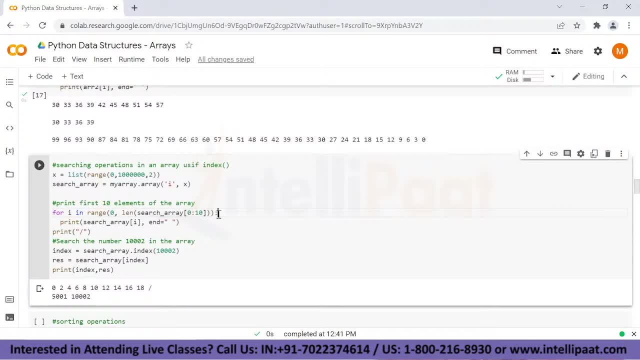 operations. we will also learn about how you can actually search for elements or you know a few searching operations using the index method. so we have a list over here which is in the range zero two i think. this is more than a hundred thousand, and we have a step of two over here. so this is a very big array, or a list which we have. 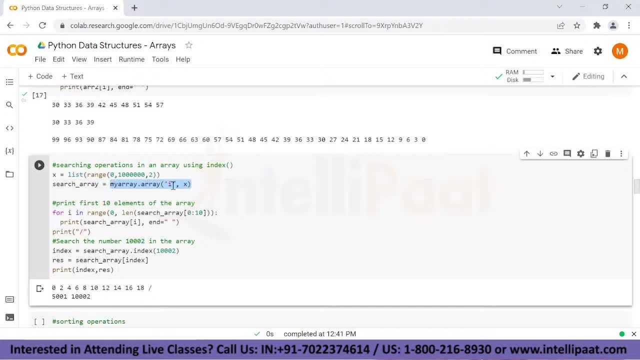 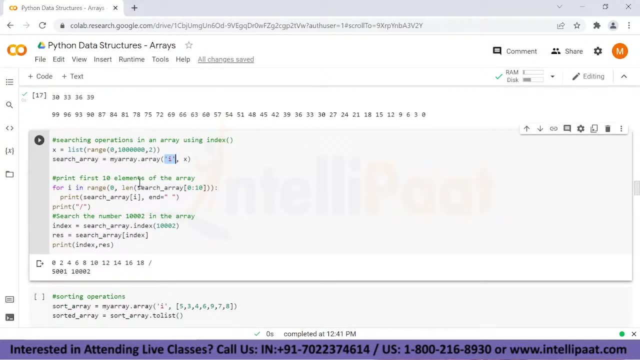 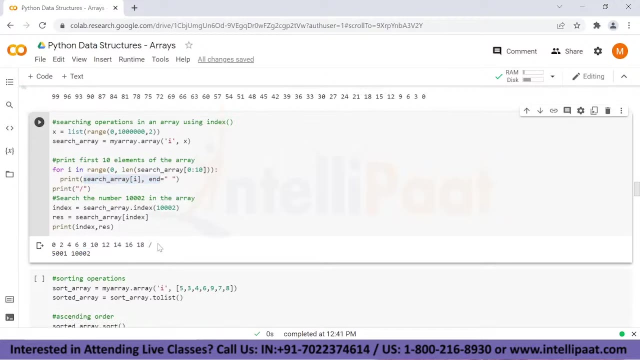 created into an array using the python array module and the type code is i, so these are all integer values. now what we have to do is: uh, let's see, we are printing the first 10 elements of the array and we are good to go. so these are the first 10 elements of the array. so these are the first 10. 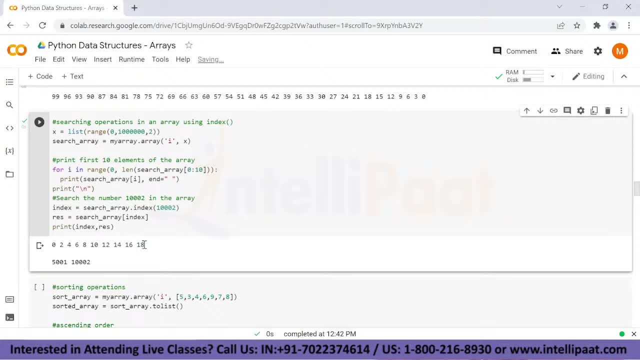 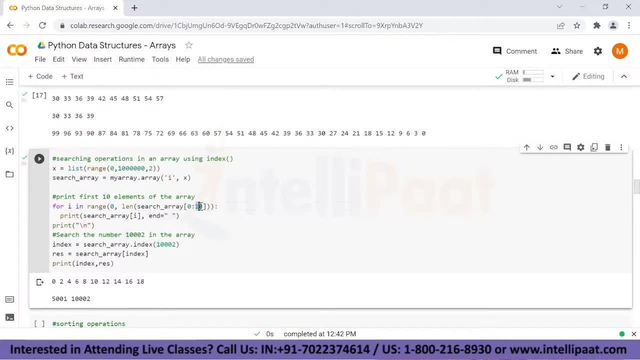 elements of the array, starting from the 0 index and going until the 10th, and you will notice that. one more thing i forgot to tell you guys: whenever you're giving the ending index over here, this will not be included in the result because it will only give the values starting from the 0 index until 9. 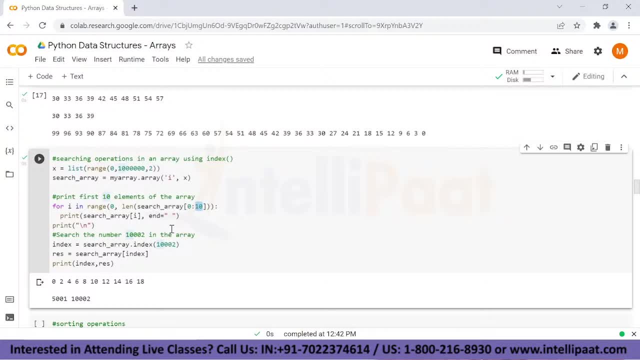 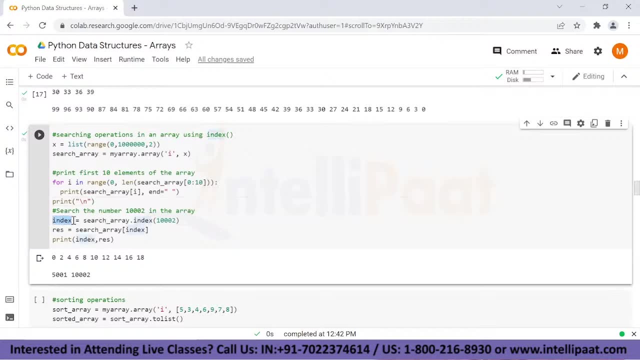 so when it comes to 10, that's where it stops and does not give you the result from over there. now coming back to the searching operations, so we are basically searching for the index which we want. basically, let's say, this is the value we want to be searched for. we get the index from using the. 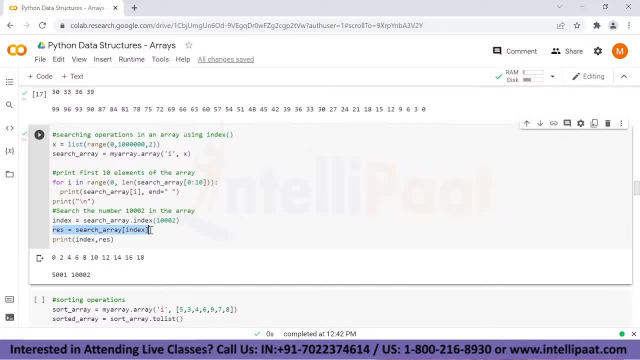 index method, which is uh, we are using to search for the array. so if you already know what we are searching for, we can get the index and using the index value, we can get the element out of the array. so this is how easy you can search for any elements using uh, the index method, in the python. 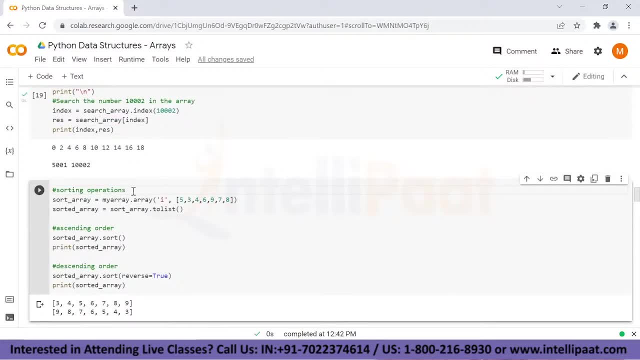 array module. now, after this, i have listed down a few sorting operations as well. where we just sort the entire array into essentially the index values, it would acknowledge the range item as time. asaki, by logging in the limit element, works for any kind ofupermode delt. this way we can generate: 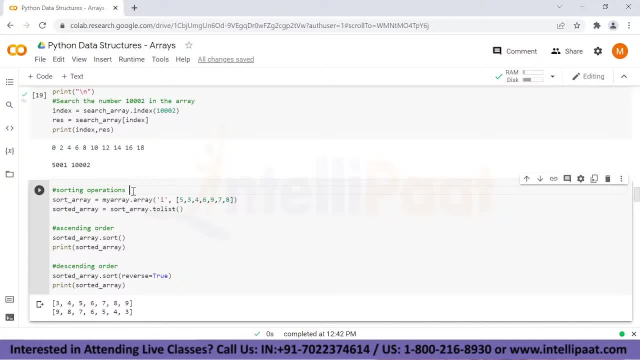 descending values or descending values, depending upon how you want your elements to be placed at. We will basically use the list methods, which is sort, and that is going to sort our array. So we have a sorted array over here. we are using the sort method and when we print this, 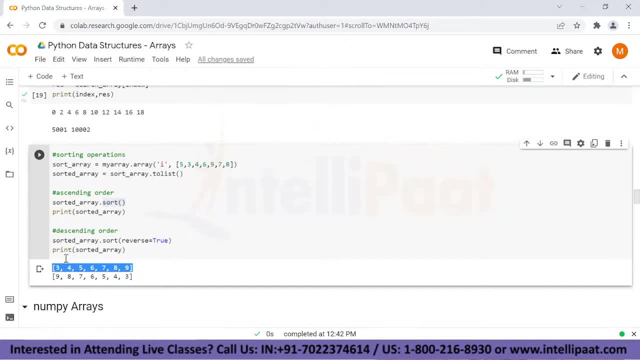 so we have sorted this into a ascending order, and if you want this to be a descending order, we will just type: reverse is equal to true in the sort method and we'll get the descending order as well. So this is how easily we can perform these operations like sorting, searching and all. 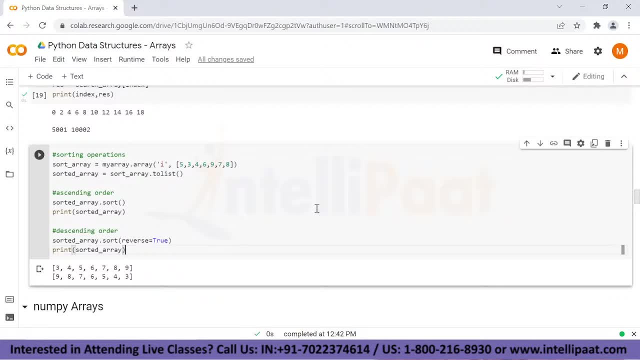 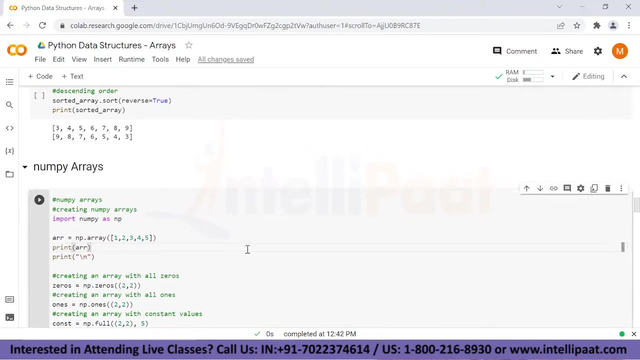 these: adding elements, removing elements, creating the array or updating the elements and deleting elements as well. So this is all about the Python array module that we already have. Now, coming back to the session, we will discuss the NumPy arrays. So NumPy, I am sure most of you must be aware of, is a Python library and it basically comes. 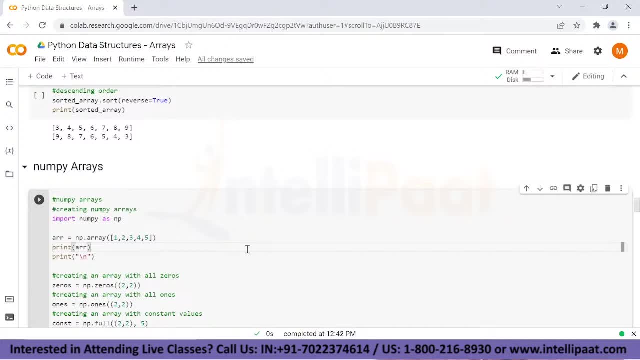 up with built-in modules that helps us with computations. So Python array are also one of the functions- or you can say modules- that it actually helps us with, and we can use NumPy for that. So, basically, first of all, what we have to do is import array and we are using np as. 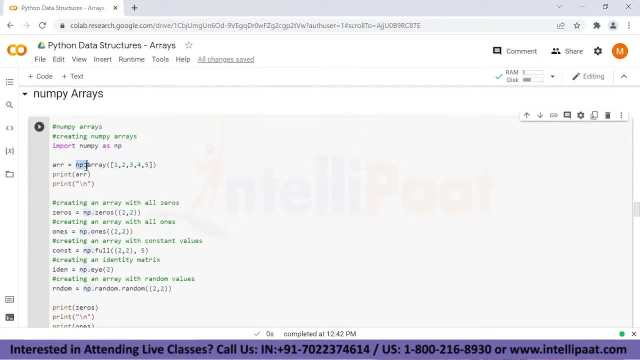 the alias over here To create an array. we use the alias np and array module and before we were giving the type codes inside here we don't have to give any type codes, it will just figure it out itself and we are just using this list of five elements: one, two, three, four and five. 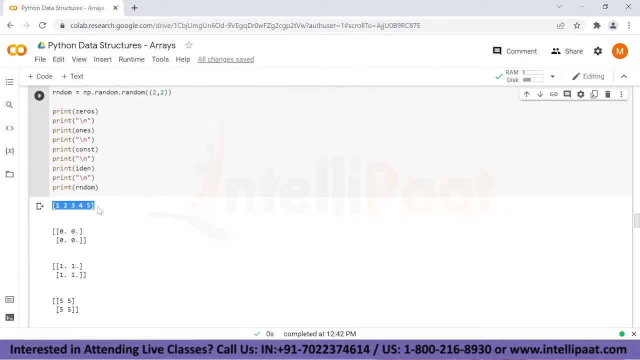 and when we print the array. this is how we get the array as So. this is as simple as creating any list, and it actually helps us with creating, you know, custom arrays as well. So here is a part where we create the array of two by two, the shape two by two, and which. 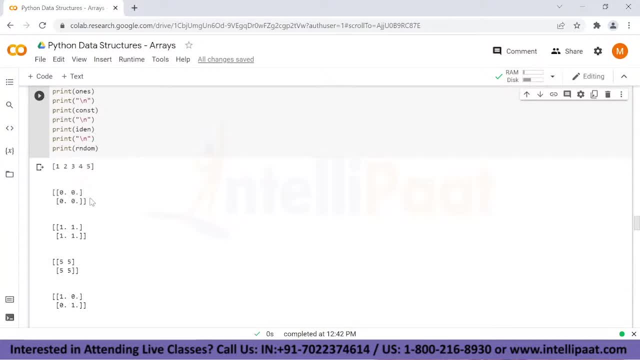 is basically all the zeros, a two by two array, and which has all the values as zero. and then we have another method once that will create a two by two array With all the values. that will be one, and you can also notice that all these values are. 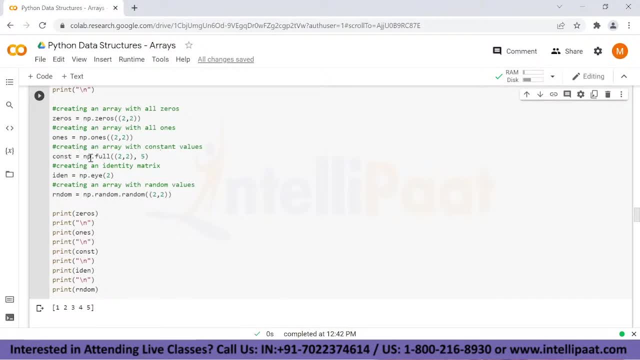 floating point values. After this we have a function called full which is basically going to create whatever shape we are providing over here. Let's say, if I provide the shape as three by three and we want the values of the constant that we want inside that array to be five, 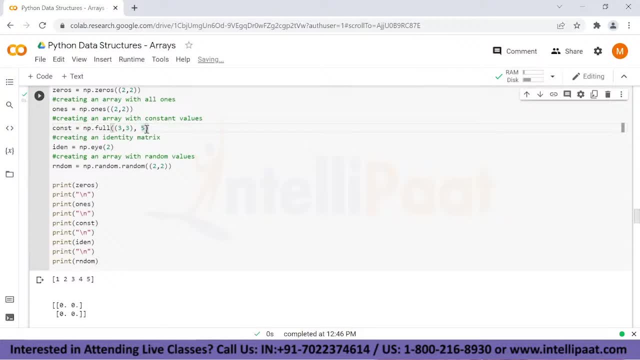 So this is what we get: a three by three array with the value five all over as a whole. So this is what we get: a three by three array with the value five all over as a whole. This is what we get: a three by three array with the value five all over as a whole. 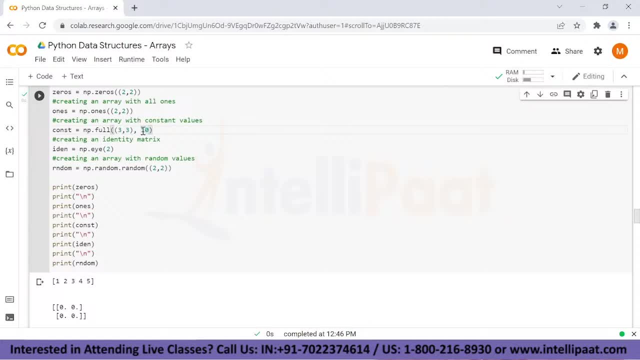 We can use two data. we can also print over here as a constant- We can do this as ten- any constant value that you want to print over here Now. after this, we can also create an identity matrix, which is basically the I method, and 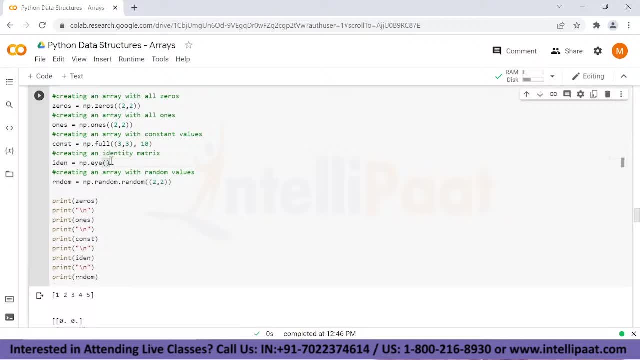 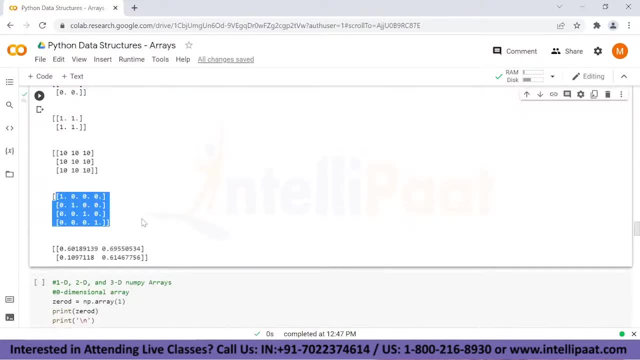 inside this we just provide the number like two in it. This is going to provide identity matrix with the two by two shape. Then we have a three by three shape. We can just decide with which kind of shape you want with our identity matrix and identity. 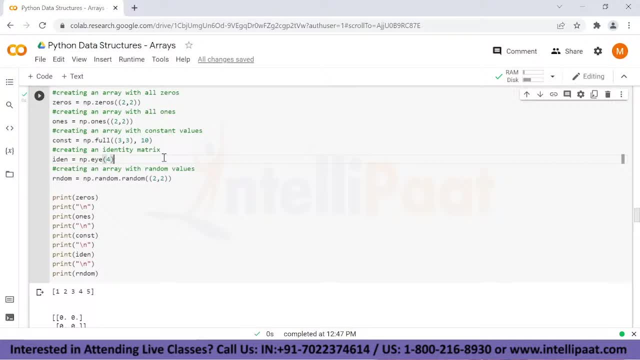 matrix is basically a very useful concept. you are further down learning about dimensionality reduction and you know principal component analysis or time series forecasting. that are these are some of the very important machine learning concepts and they make use of linear algebra and in linear algebra you'll come across identity, matrix and 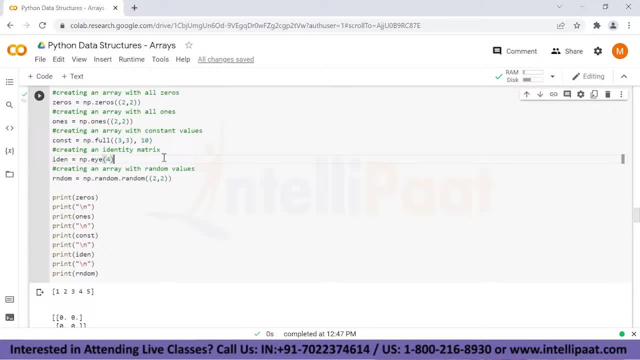 arrays of different shapes and sizes. there you will be handling dimensions to be, let's say, four, five, fifth, and that that's how you want to learn linear algebra using numpy arrays. so after this, we have another method which basically creates array with random values. so this is how you simply create it, just give. 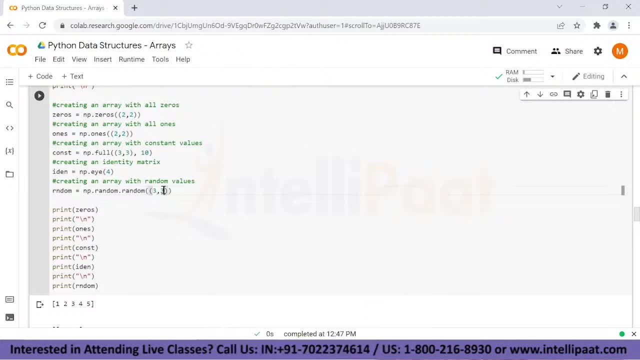 out the shape and it will create the array with random values: a 2 by 3 or a 3 by 3, depending upon your requirement. you can just create random arrays with the random values. so these are a few operations, how you can create the numpy arrays. so we 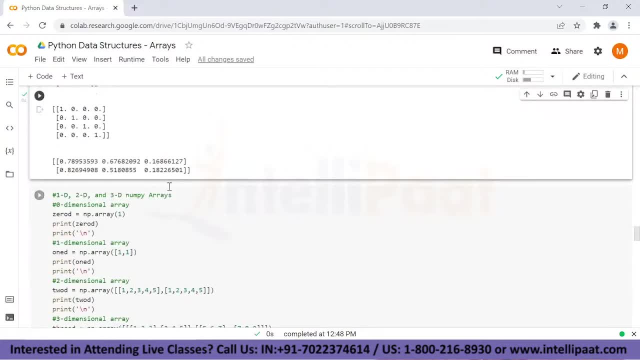 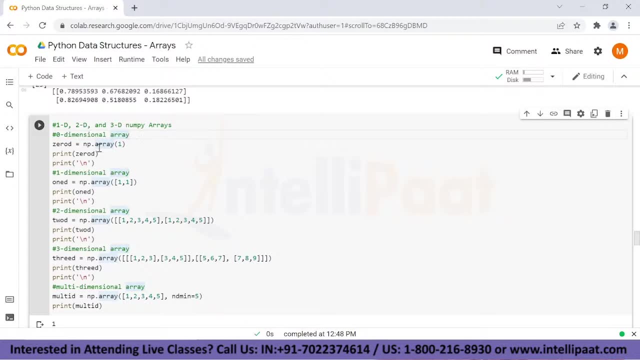 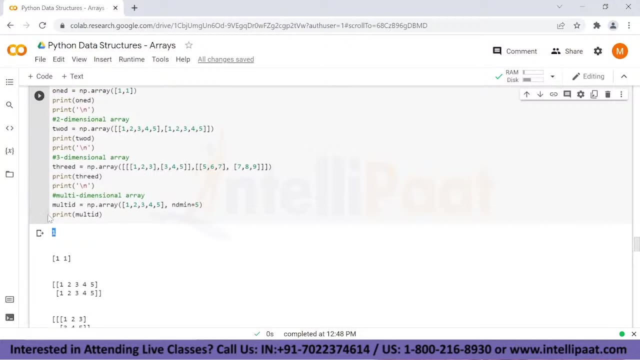 already covered how you can create the numpy arrays. let's take a look at how we can. we have multiple dimensions that we can use with the help of numpy arrays. so this is how you create a zero dimensional array: just provide the scalar value over here. it will create a one dimensional array like this after: 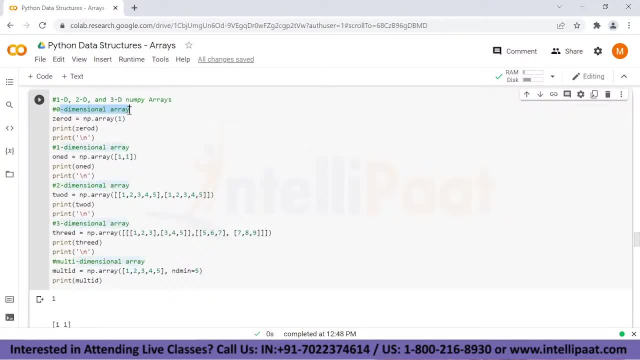 this, you create- I'm sorry guys- a zero dimensional array. that's how you create a zero dimensional array. for a one dimensional array, that's how you created, and for a two dimensional array, you have to create a nested list or a nested array, basically. so that's. 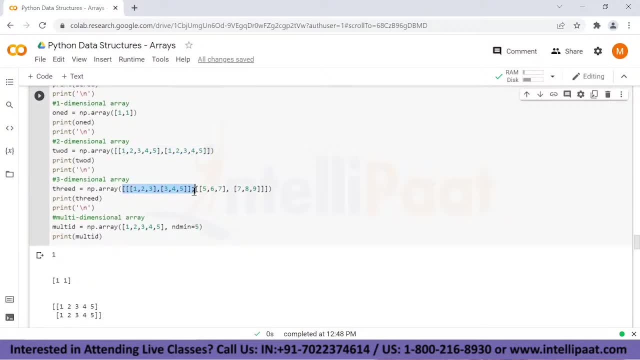 how you create two-dimensional array and for the three-dimensional array we have a two-dimensional array nested inside of area. so basically, a three-dimensional array will consist of, let's say, for example, two or three or maybe four two-dimensional arrays. so now, here we have a. 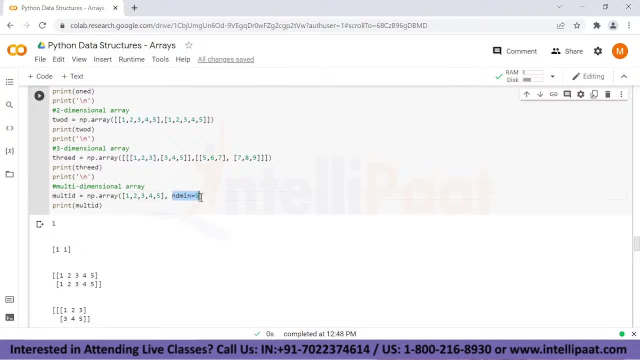 another parameter called and dimensions, where we basically provide the dimensions. So if I wanted it to be a two dimensional array or a three dimensional array or multiple dimensional array, this is how I can assign the values and get the resultant array. So now that we have covered creating the array using NumPy, let's let's take a look at how. 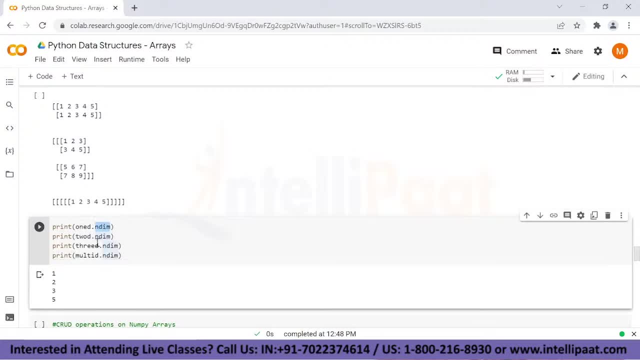 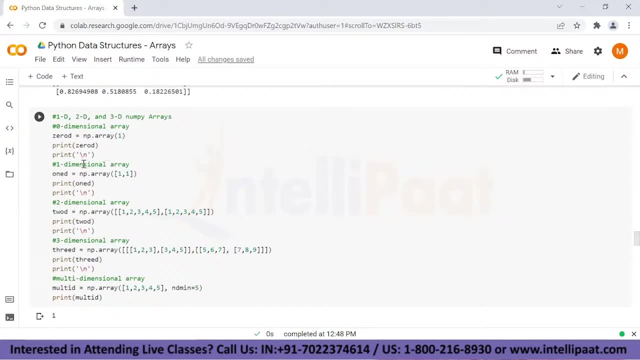 also, if you have created all these arrays, you can check how many dimensions it has using the n dimensions method. So this is how you get the values as. so the first one, we're getting it as one dimensions, And similarly for the ones, we're getting the same for a zero, zero. 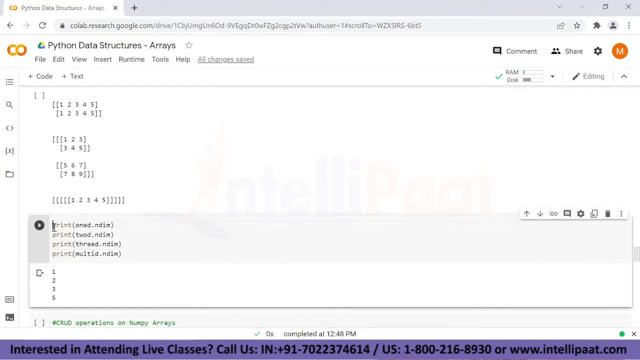 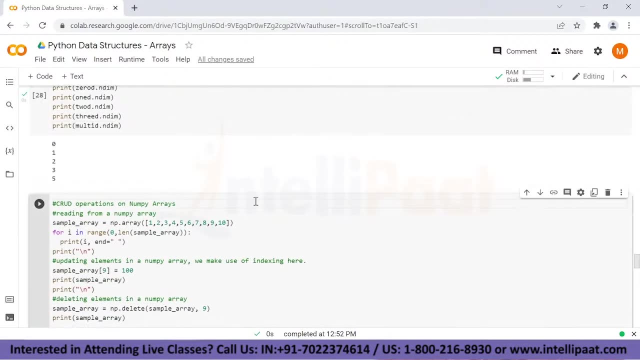 dimensional array. let's just check for the zero dimensional array as well, if we can get the value. So we're getting that dimension as zero again. Now, moving on, let's understand the other operations that we have on NumPy arrays, just like we have done for the Python. 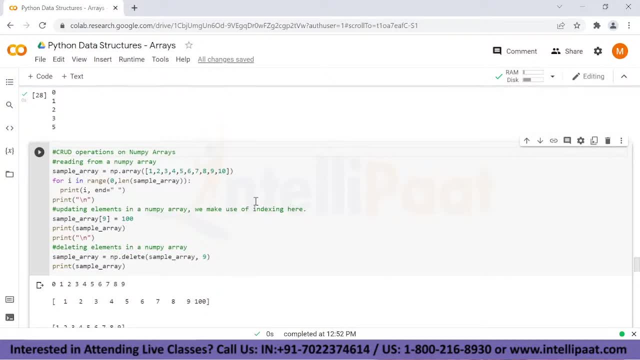 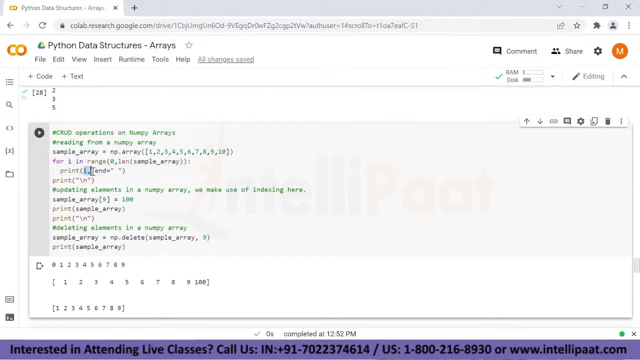 array module, like how we access the elements, How we update the elements, how we remove the elements and so on. So, reading from a NumPy array, we can use the same approach we're using for the Python array moduli. we using the for loop, inside which the range is basically the length of the array, And then we print. 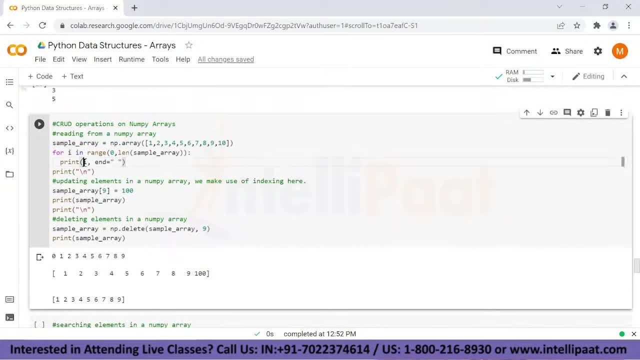 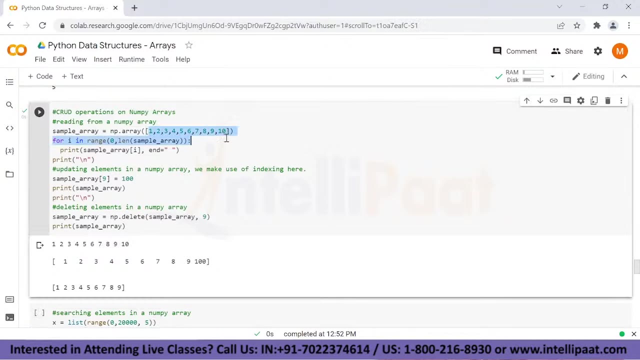 the values like this: So we're getting all these values again. All right, so I think we have made a slight error here. we forgot to give the indexes, And now let's see if we are getting the values again. yes, so we are getting the similar values from the array, and that's how we 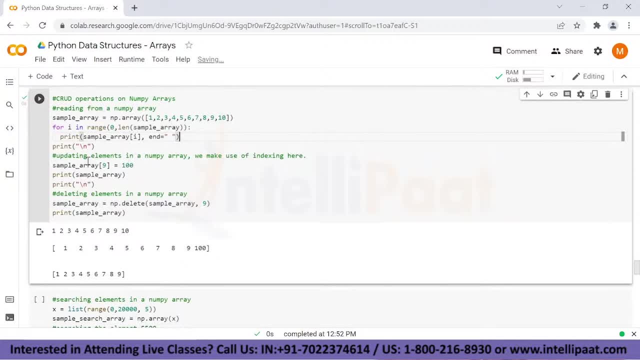 read from any nympy array, just like we have done for Python arrays. now updating the elements again, we use the same approach: if we already know the index value, we just use the index value and update the value. if we don't have any values regarding the index, we search for the index value for that particular. 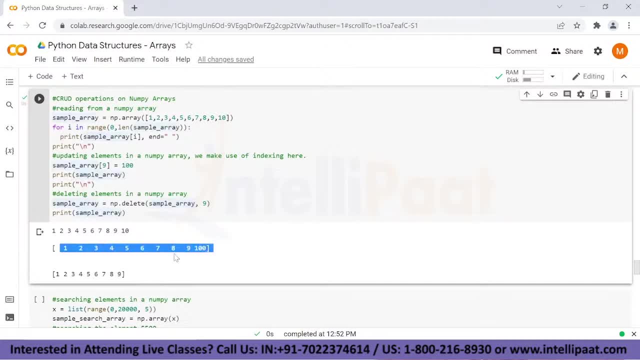 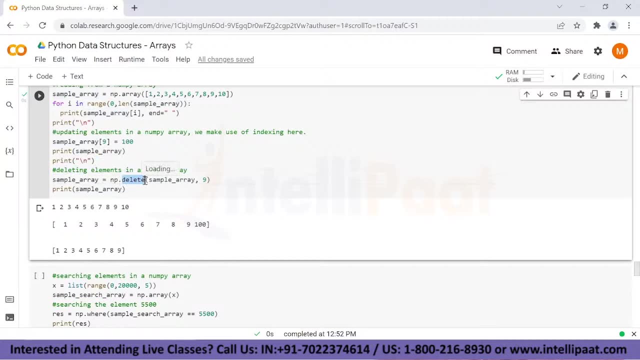 element and after that we can update value. so this is how we have done that and now, after this delete the element again, we can use the delete method we have from numpy, so we don't have to use the pop method in any other methods. we can just simply provide the data we are deleting from and the index value. so 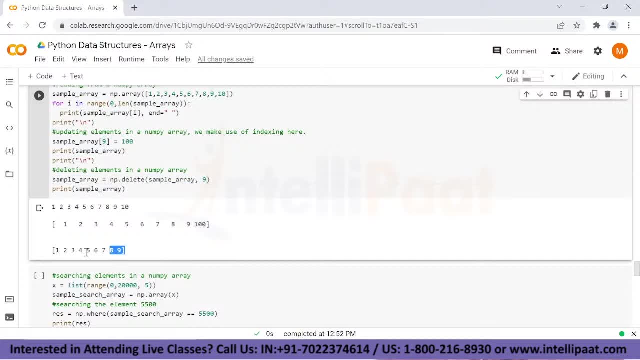 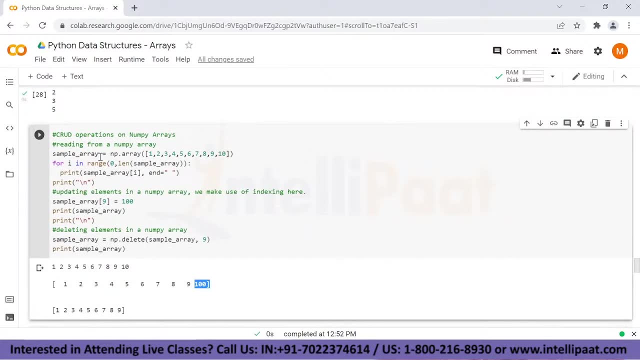 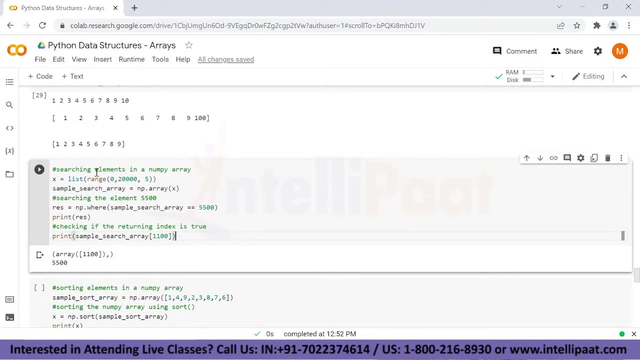 since we are removing the ninth index, so we are getting the resultant array as this. so the last element has been removed. so the cred operations are creating, reading, updating and deleting elements from an umpire. we have already covered how we can search and sort from the numpy arrays, so searching elements in 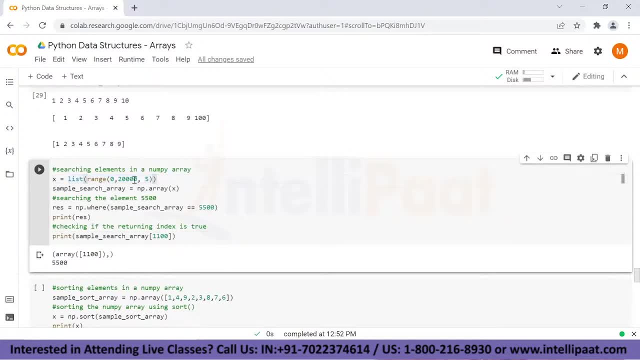 any numpy array. we are using the same approach. we have a list over here which has all these values, 20,000 values, with a step of 5. so we have a sample search array we have created using the numpy and after this we want the numpy where. 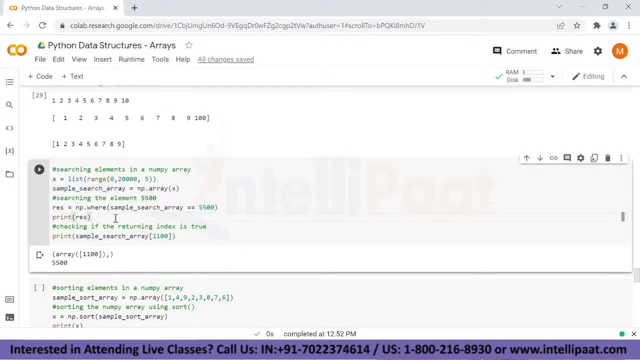 sample search array is 5500. so the difference between how you are searching the elements from the Python array module and this numpy array, we have this where method which basically helps us give the expression which we want for our element and we basically get that element and just to check if the 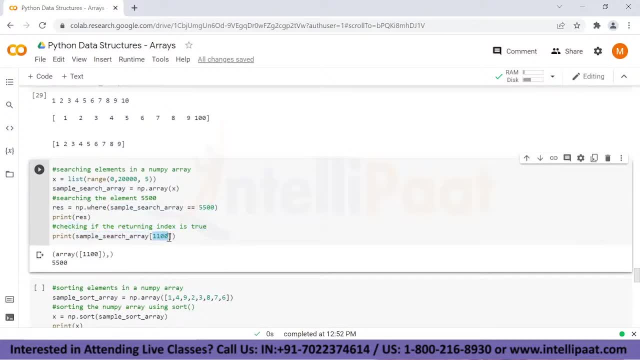 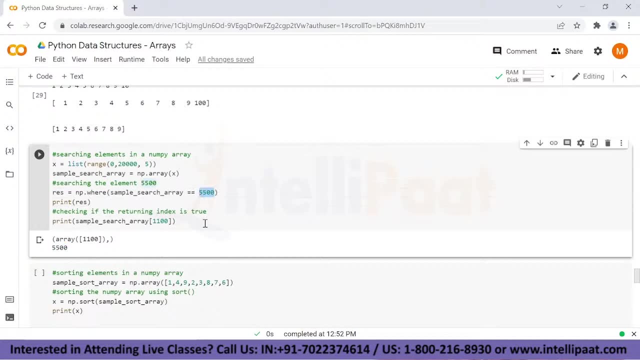 returning index is true or not, we will print the sample array at the index number, whatever we have got from the result over here, and this is how we are getting the exact same number, which means this is basically searching the element quite efficiently. now coming on to how we sort the elements inside the 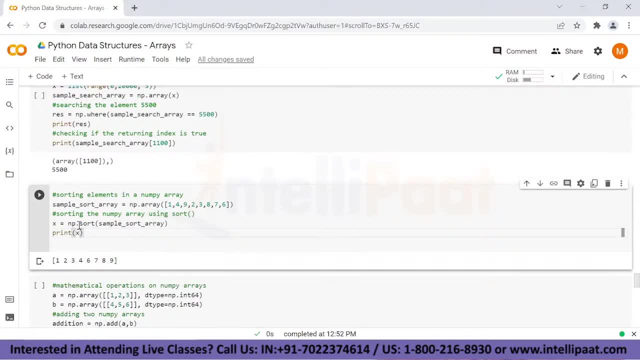 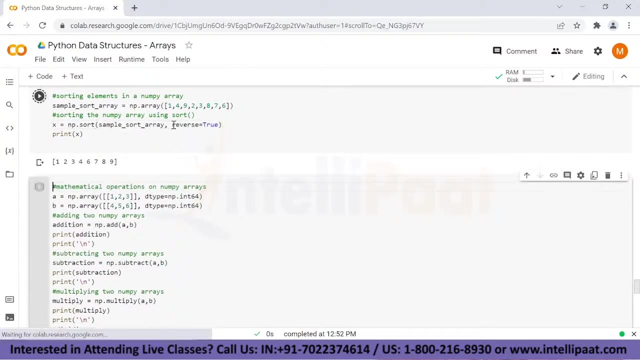 numpy array. we are using a, a again, the sort method which we have in the numpy, and it is basically sorting us the element in the ascending order. now let's see if we have the reverse is equal to true argument if we can pass over here. so sort dispatcher, gotten an. 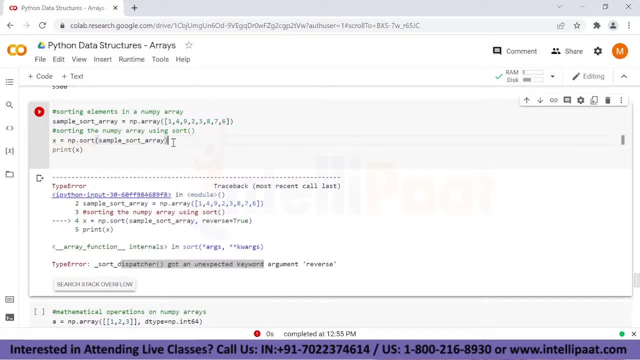 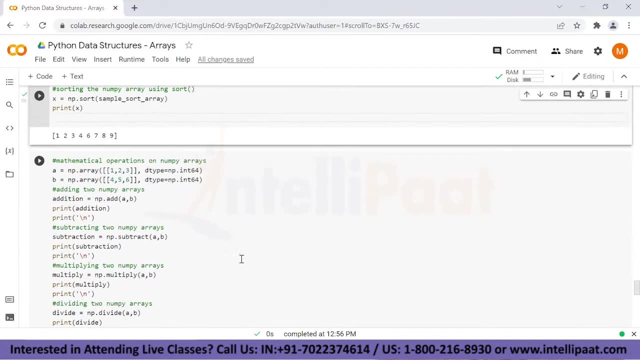 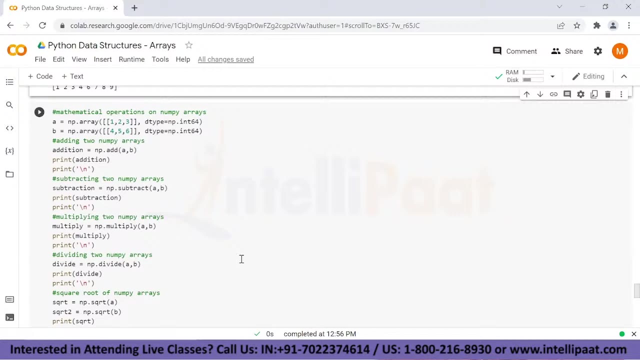 expected keyword argument: reverse. so we do not have that over here. so this is how we sort the elements inside a numpy array. now, after this, let's talk about a few mathematical operations. also, we can perform on our number ARAs, so not just the current operations we can also make use of. 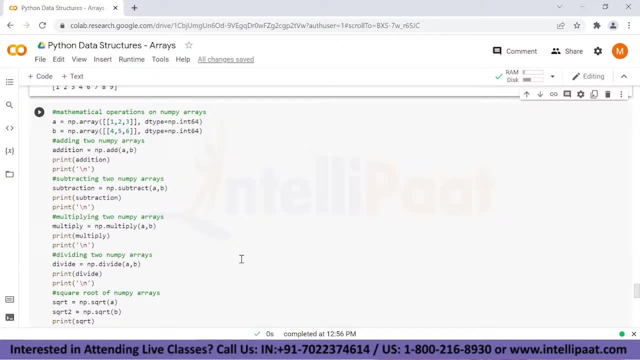 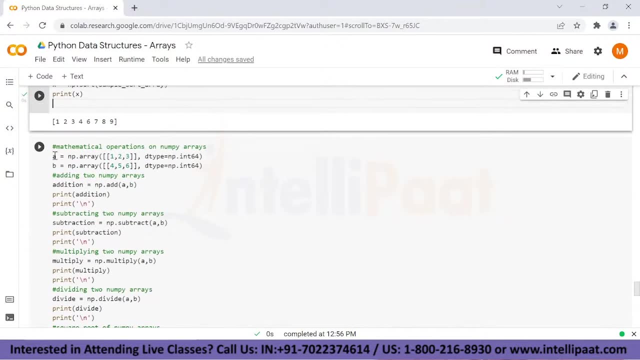 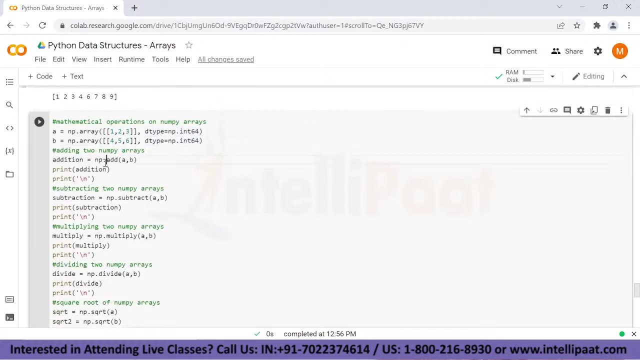 mathematical operations like adding, subtracting, dividing, getting a transpose of the shape 3 by 3 matrix and multiplying square root. so that's how we do it. you basically have these two areas which we have assigned using the datatype integer. now what to add these two numbers? we are using the ADD method over here. 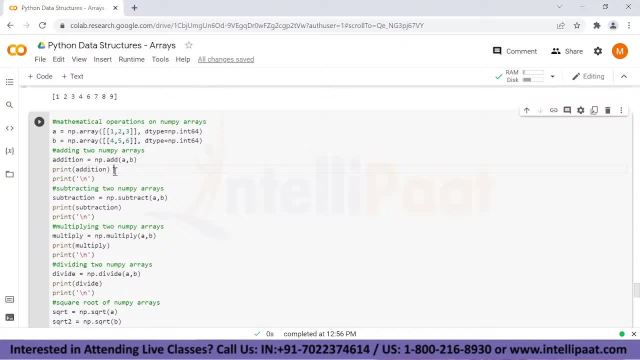 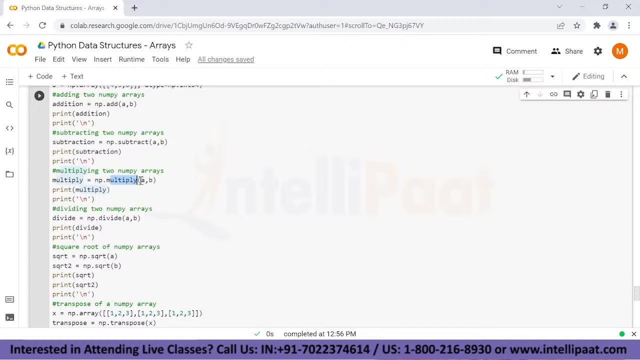 which basically needs two parameters, just the arrays that you want to add, and we get the result like this: and is that we want to subtract from. so this is how we can subtract two arrays. after this, we have the multiply method, which basically also has only two parameters. after this, we have the divide parameter, which we 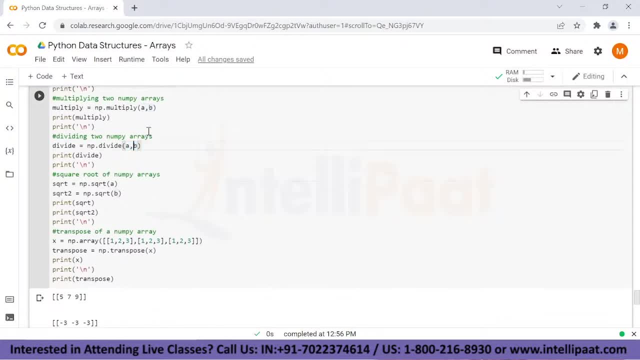 has the two parameters again which we want the number to be divided from, and after this we have the square root again. the square root method will get only one parameter. so if, let's say, if I want to get the square root of all elements from an array, I can use this method and then again to find out the transpose of a. 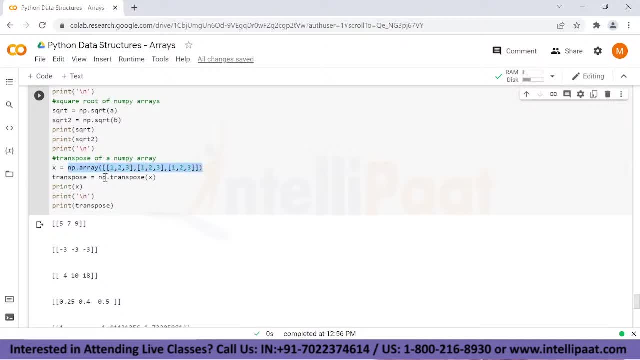 matrix. we have created another numpy array, so this, basically, is the array. now, if I want to get the transpose of this method, I'm using the transpose method, which is the parameter, and this is how it will look differently. so this is the original array that we had and this, basically, is the transpose of that particular array. 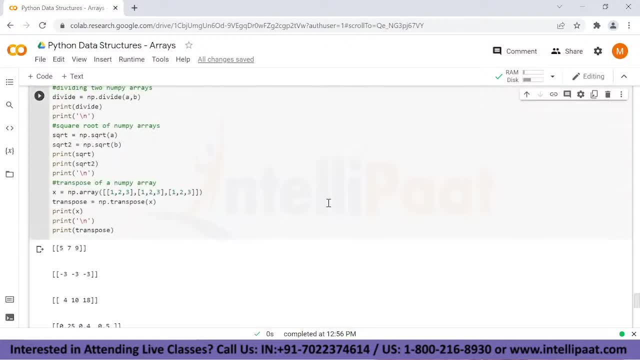 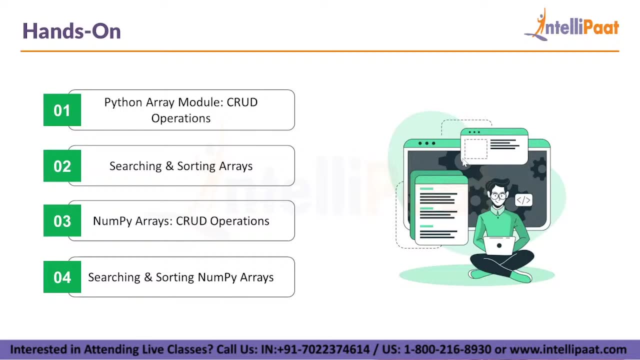 so with this we have come to the end of the session, guys. so that's all for Python arrays. so that's it for this session, guys, in the hands-on section we have learned about the Python array module: how we can create an array, how we can read, update and delete the values or the elements from the array. we have learned 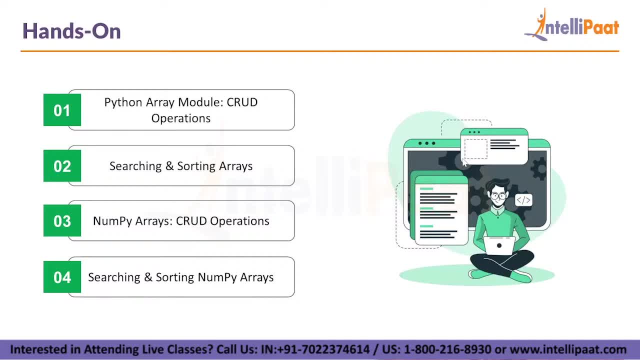 about how we can search the elements inside an array. we have learned about how we can sort the arrays of the Python array module. after this, we learned about the numpy arrays, how we can create them, read, update, delete all these values from the numpy arrays. and we have also learned 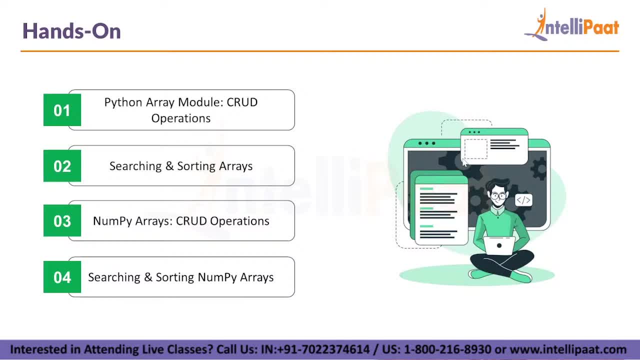 about the searching and sorting of numpy arrays. additionally, we learn about the mathematical operations that we can perform on the numpy arrays. so if you have any questions, guys, you can mention them in the comment section below and we'll be happy to help you out in your journey to learn data structure starting. 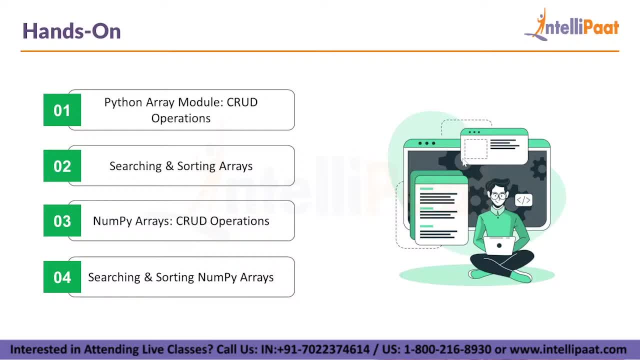 from the numpy arrays. stay tuned for the upcoming sessions on Python data structures and if you have any questions, or don't forget to mention them in the comment section below, guys, we'll be happy to help you in your journey to master Python programming. now that we are done with the session, don't forget.